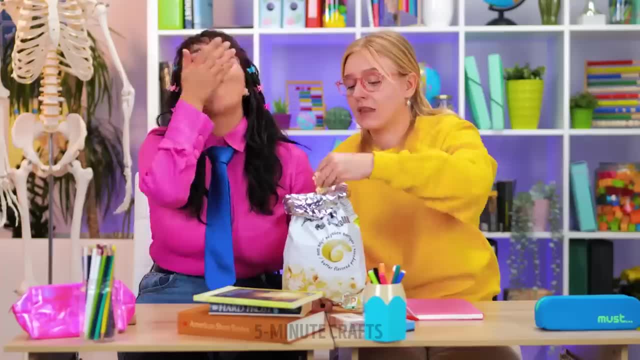 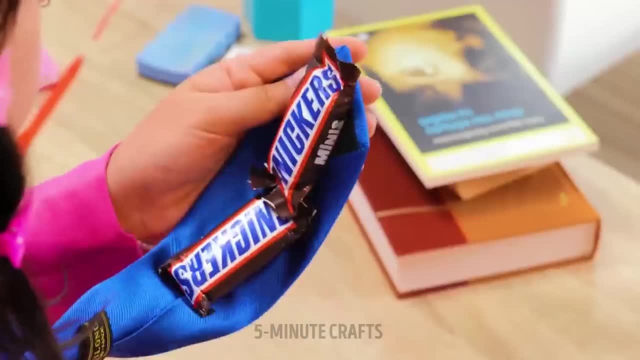 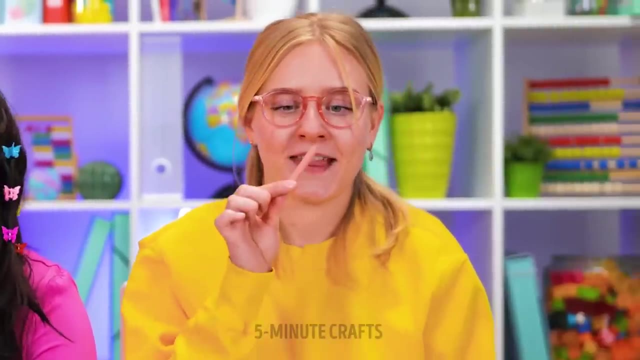 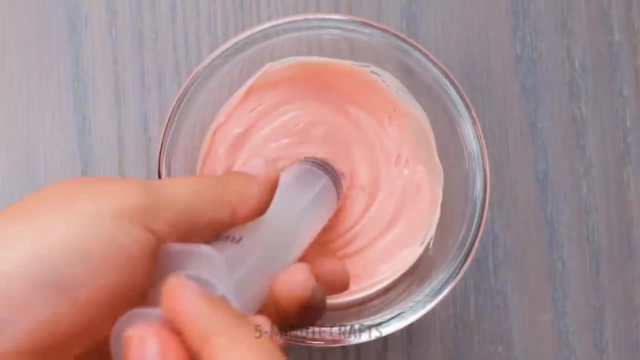 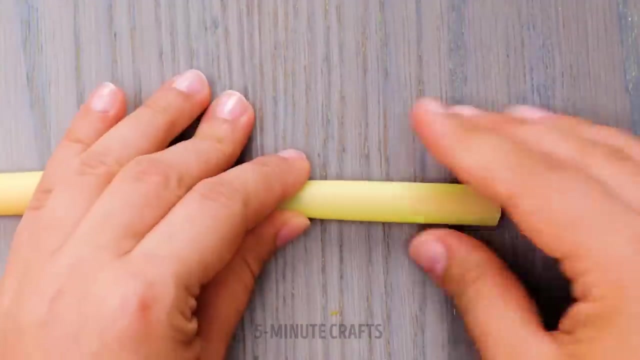 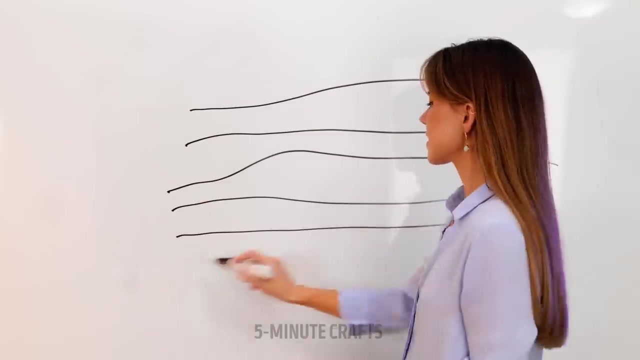 Get out your bomb and fly away. We'll be dancing With our hands in the air When our new dawn is rising To the break of dawn. We'll be dancing With our hands in the air When our new dawn is rising, Dancing. We'll be dancing With our hands in the air. 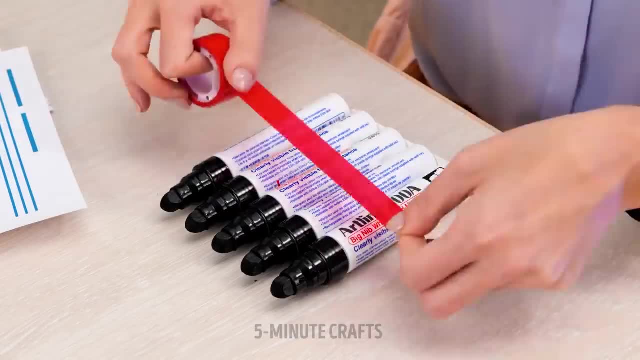 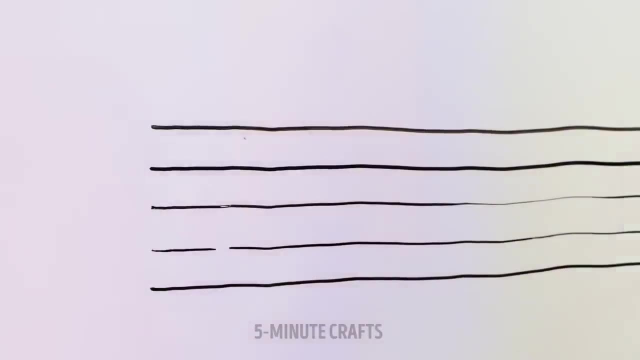 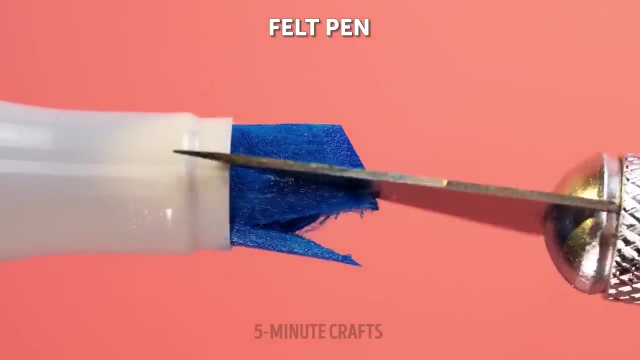 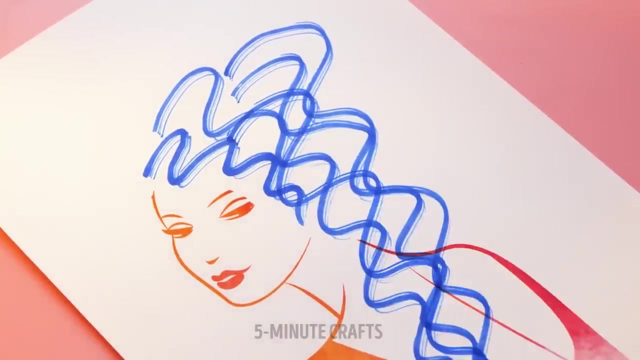 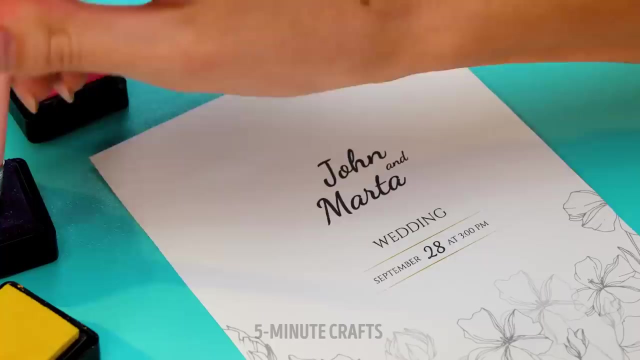 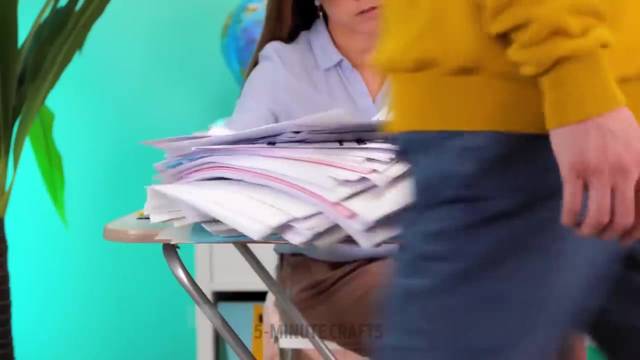 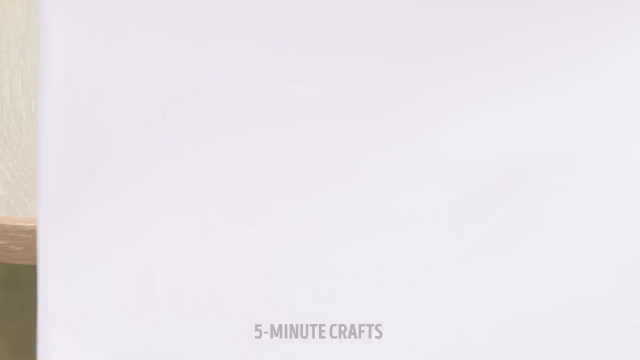 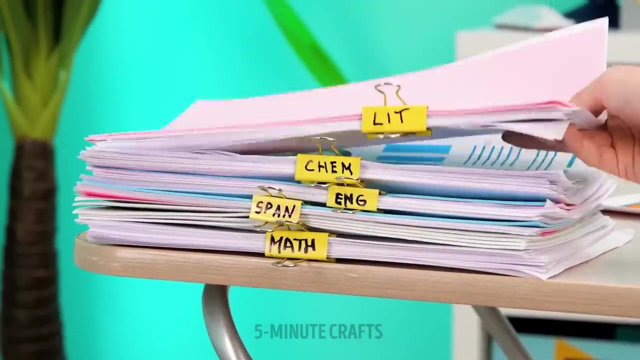 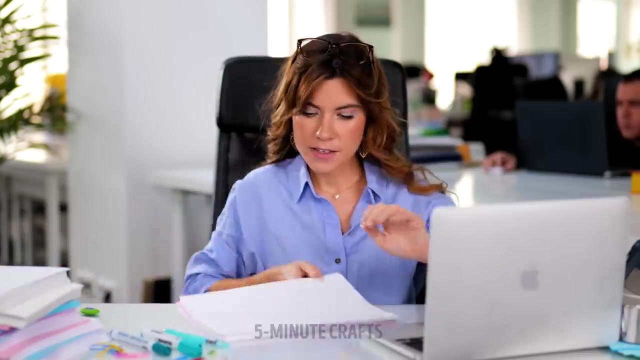 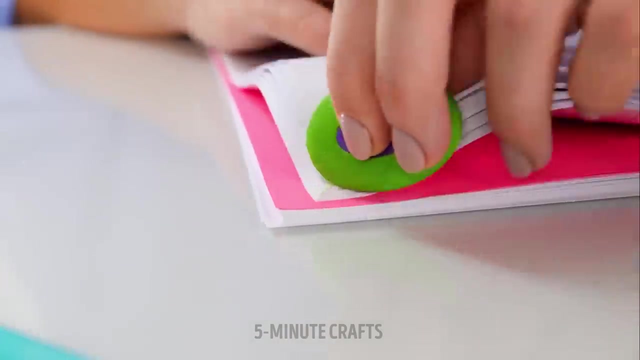 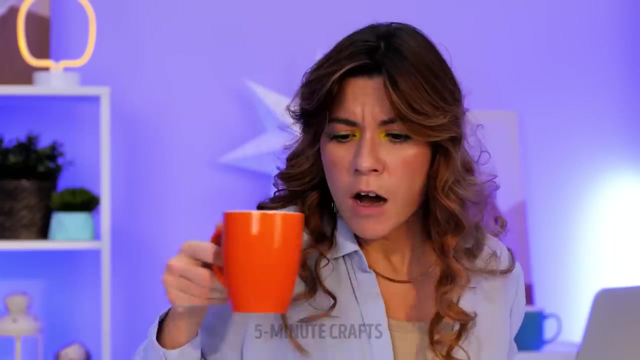 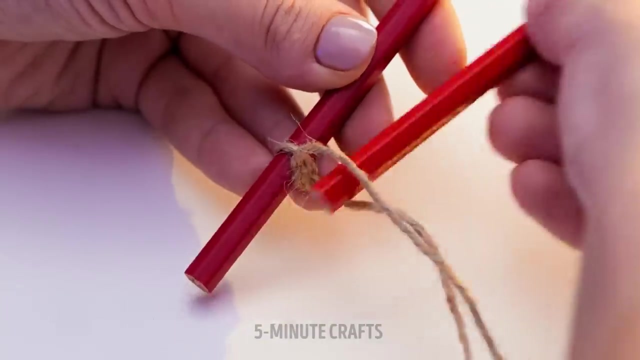 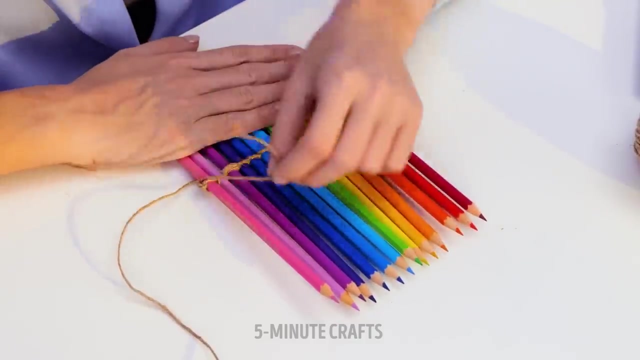 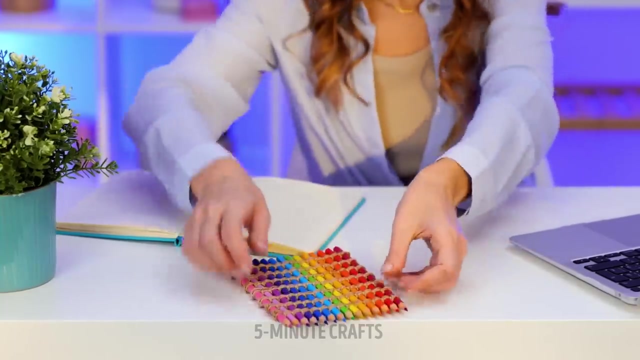 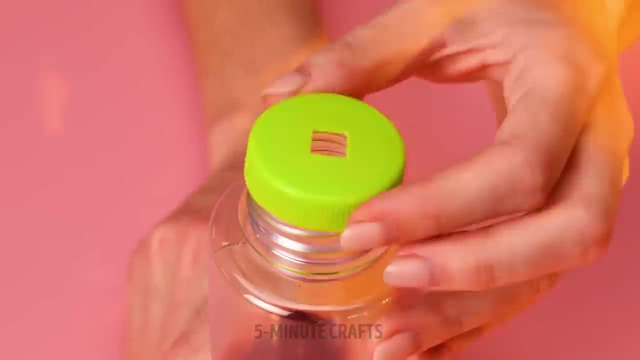 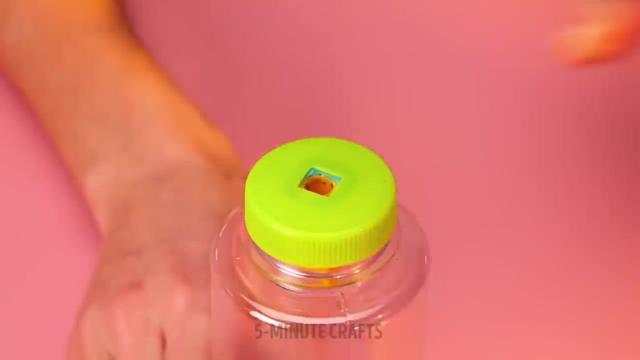 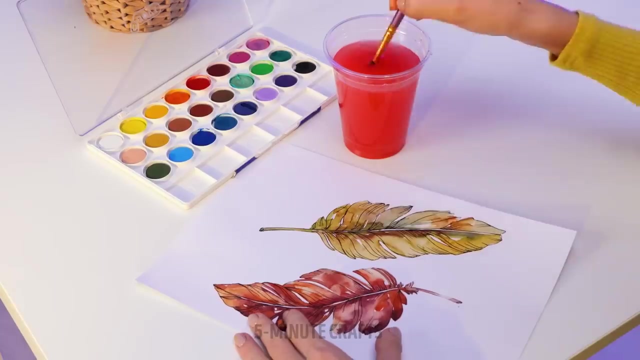 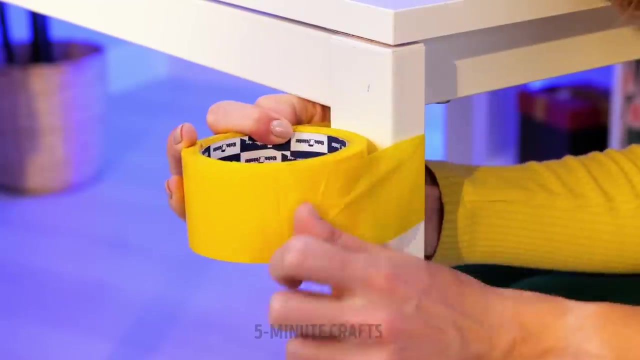 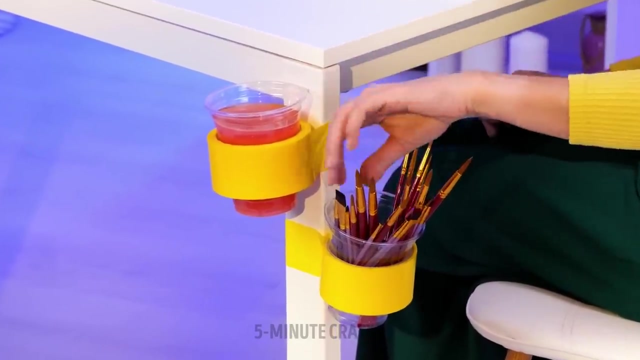 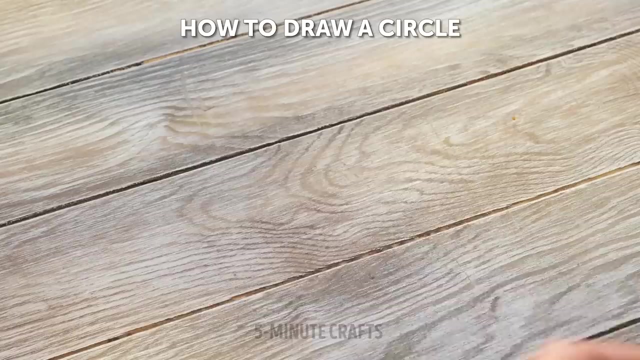 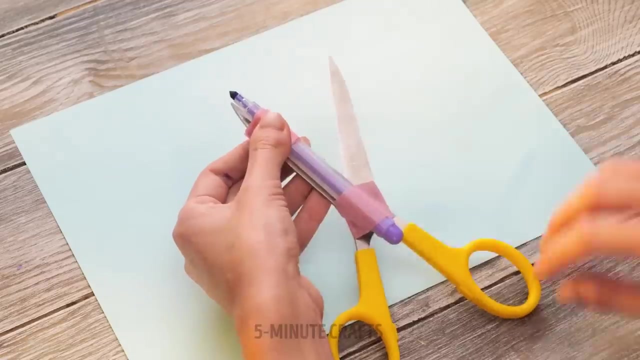 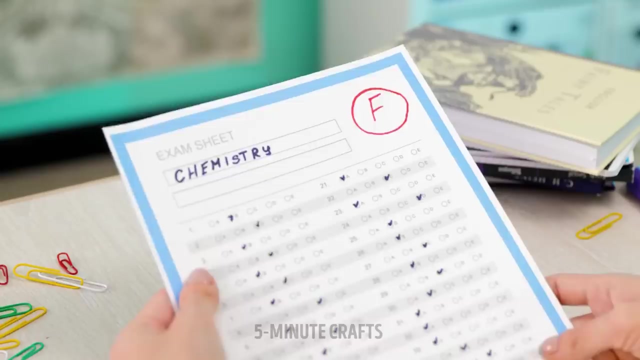 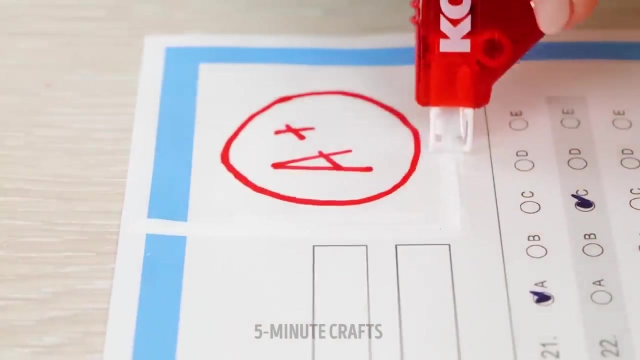 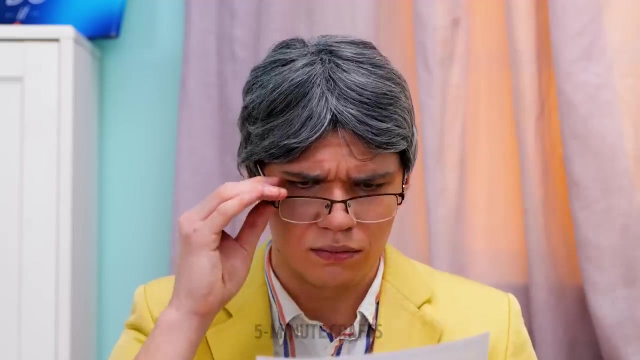 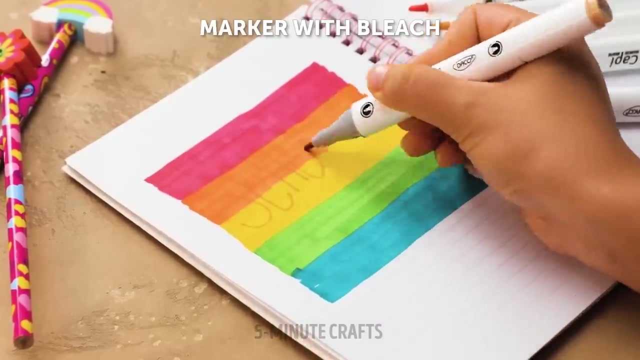 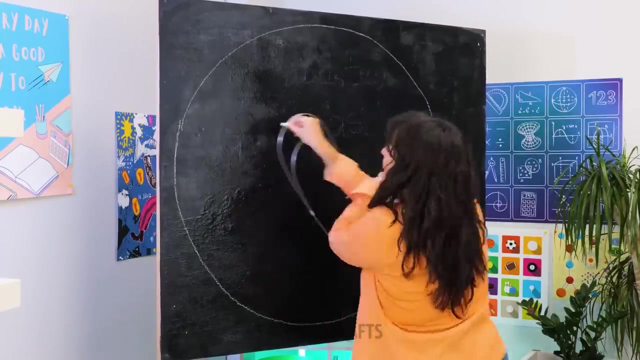 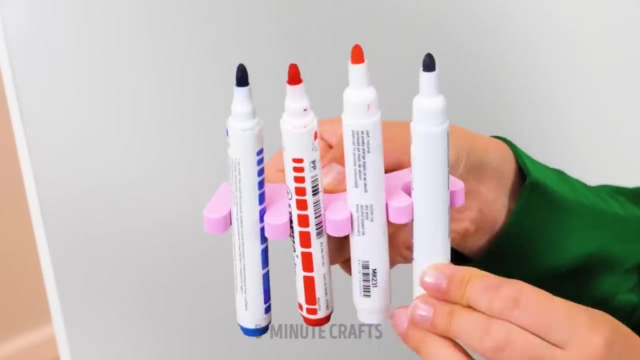 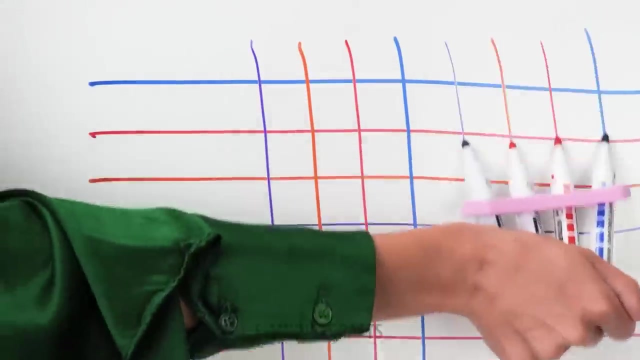 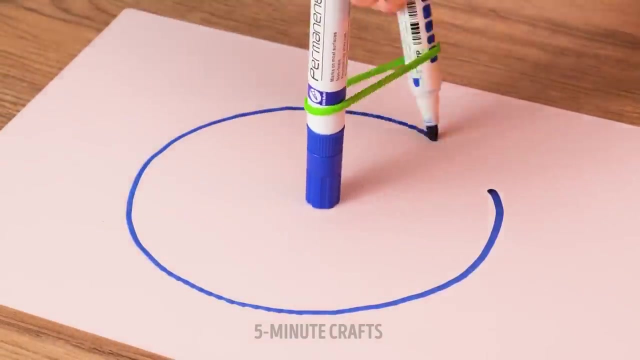 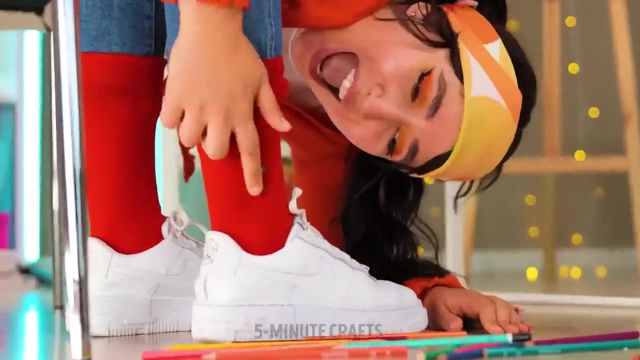 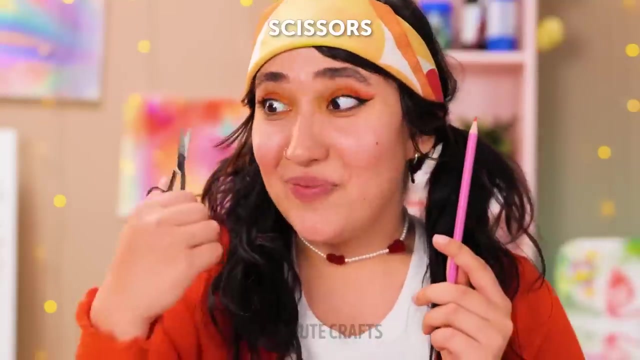 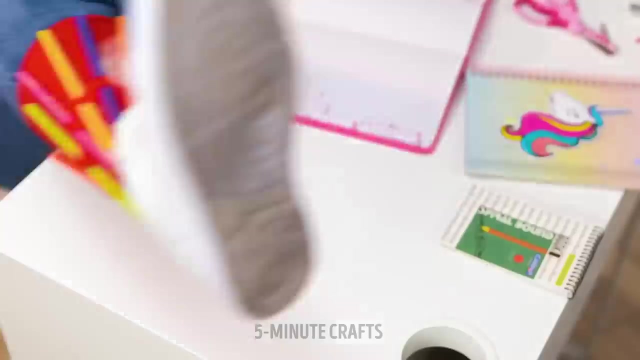 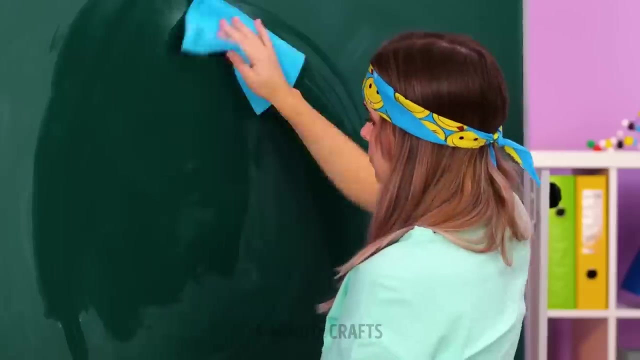 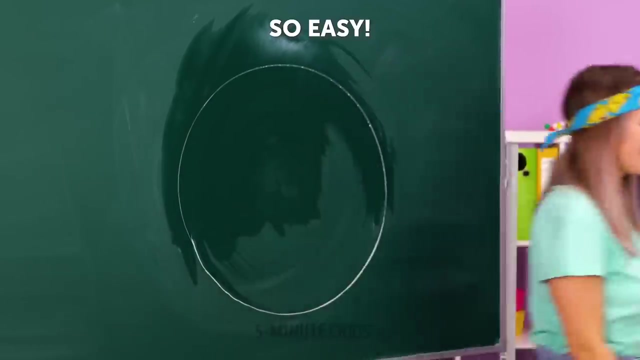 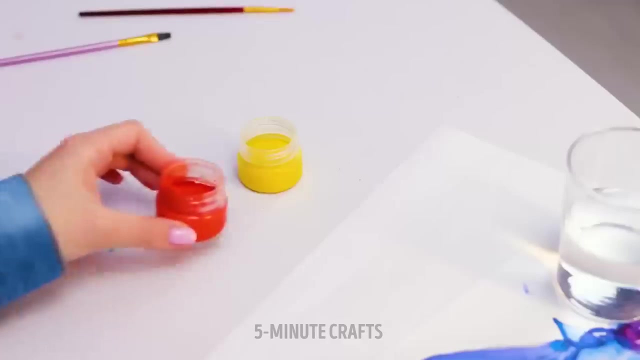 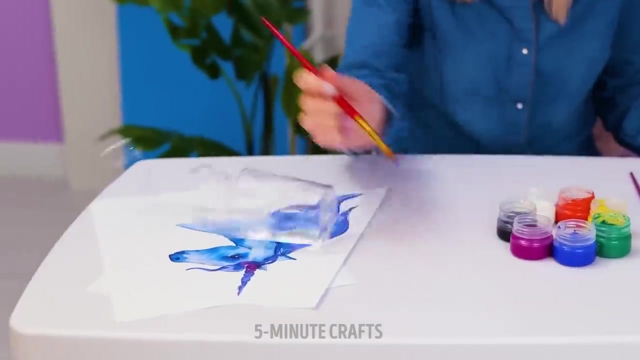 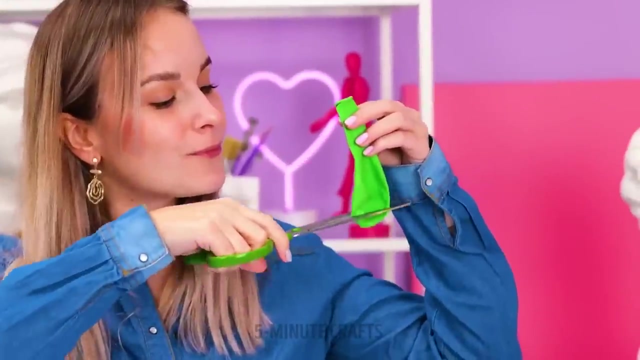 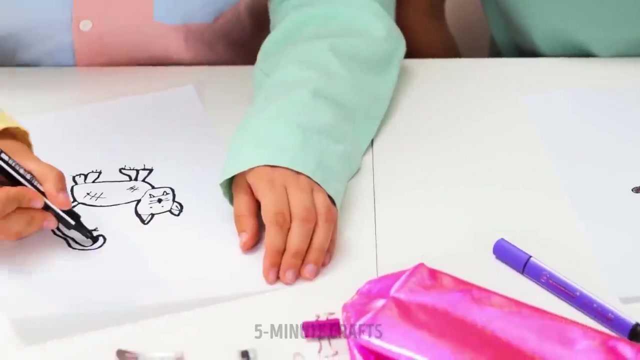 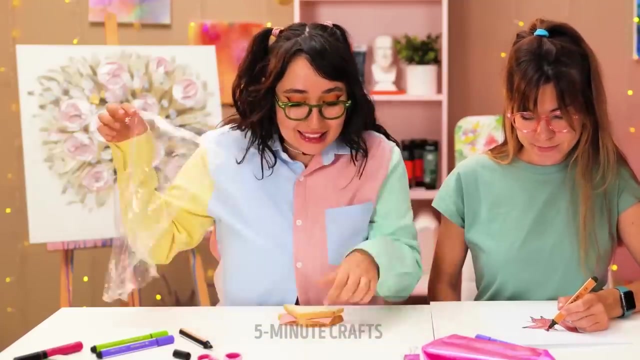 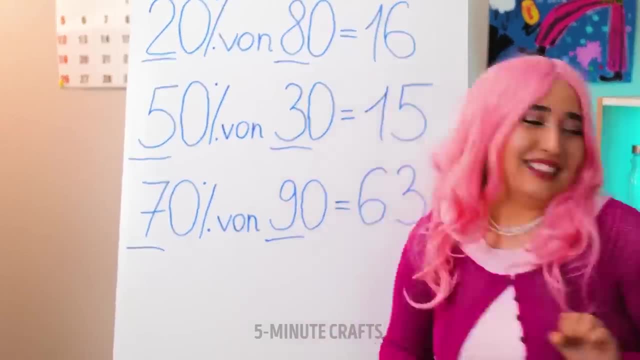 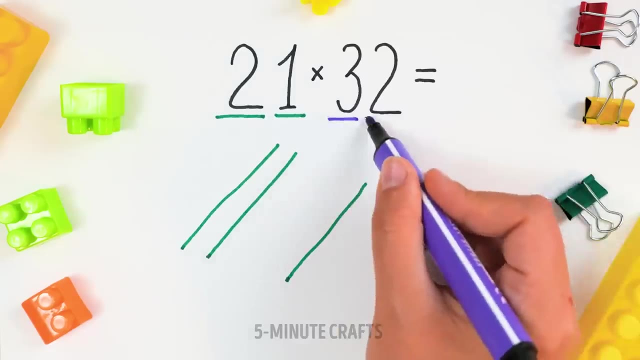 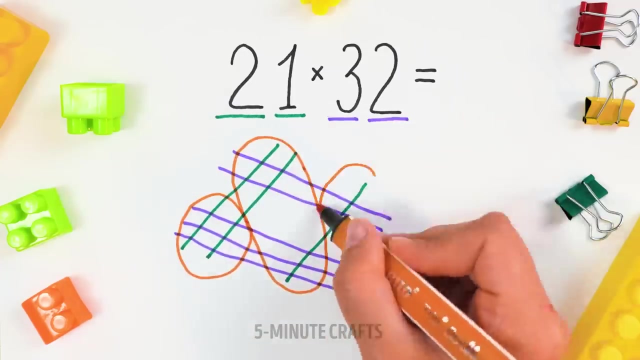 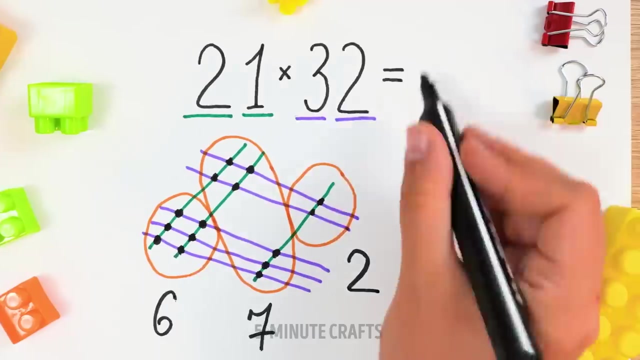 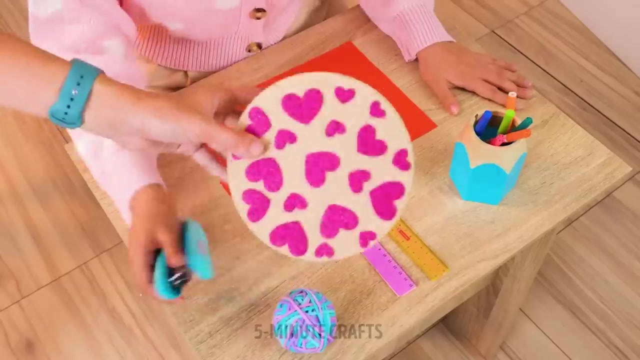 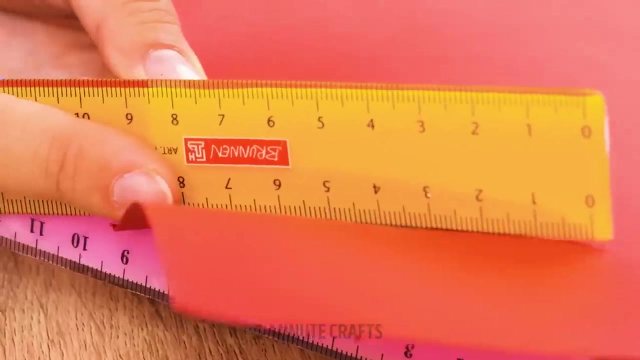 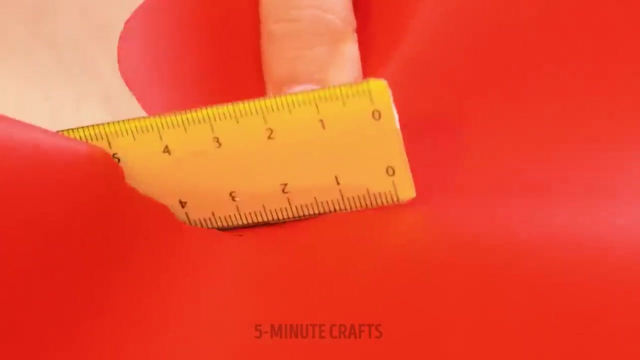 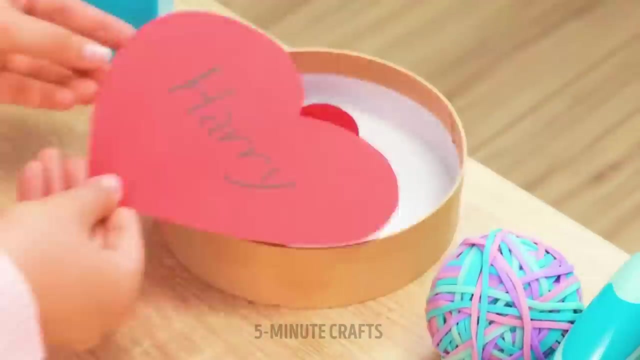 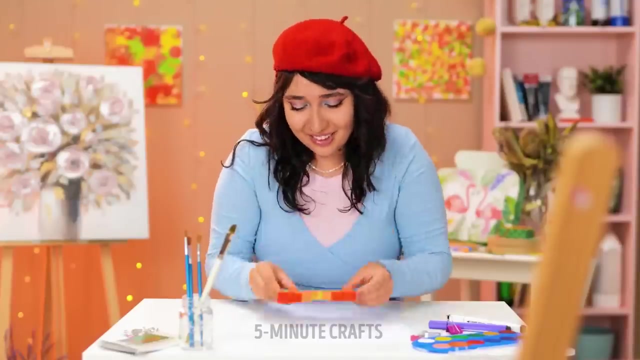 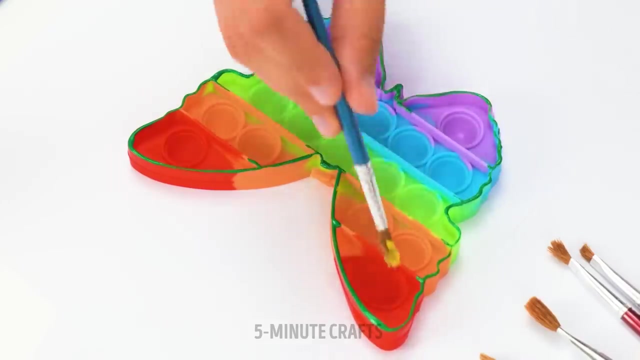 Yeah, I'm awake. I'm giving it to you. I'll do my part. Yeah, I'm awake. Did you let it go? I'll do my part. Yeah, I'm awake, I'll give it to you. Yeah, I'm awake. I'll give it to you. 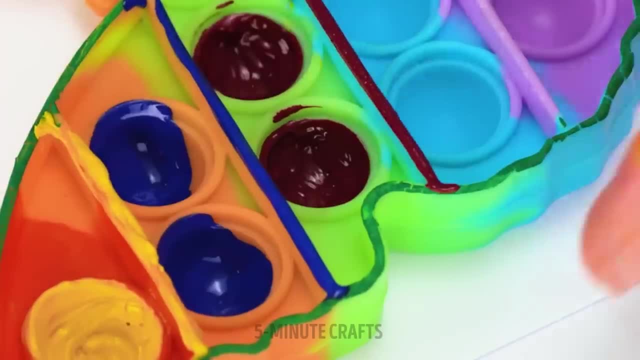 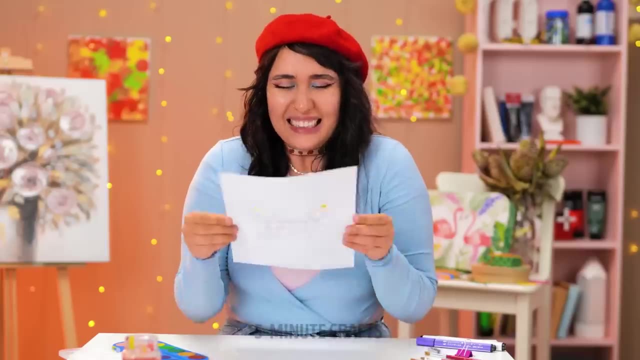 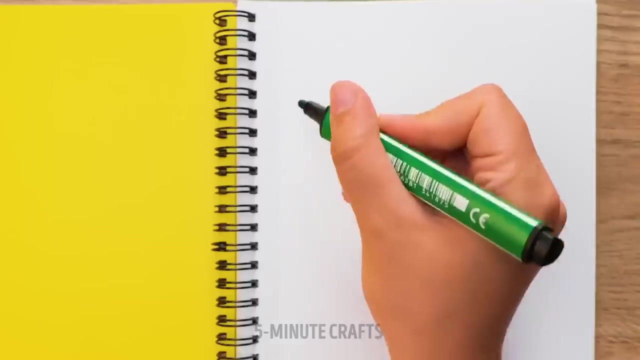 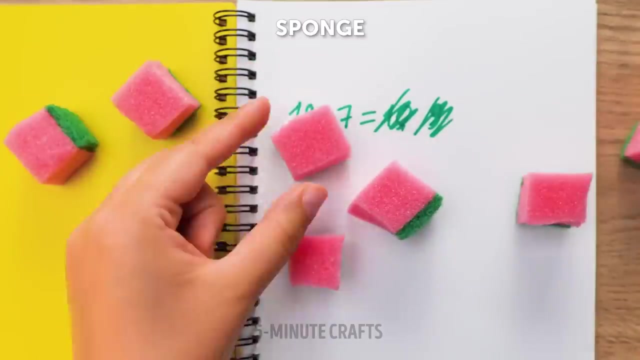 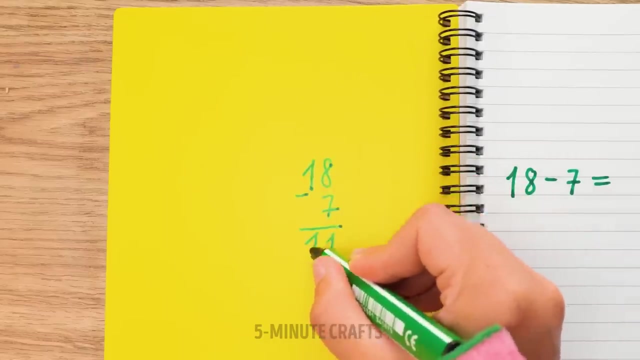 I'll do my part. Yeah, I'm awake. Did you let it go? I'll do my part. Yeah, Yeah, I'm awake. I'm giving it to you. I'll do my part. Yeah, Yeah, I'm awake. Did you let it go? Did you let it go? 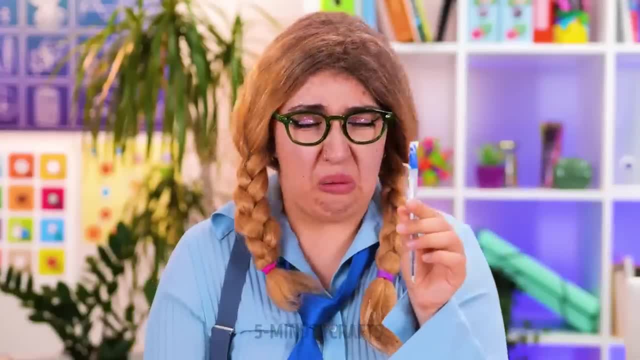 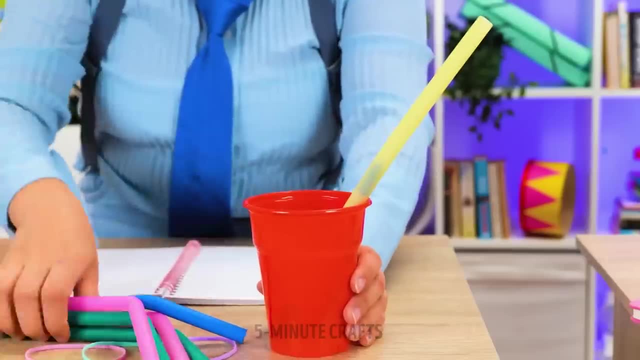 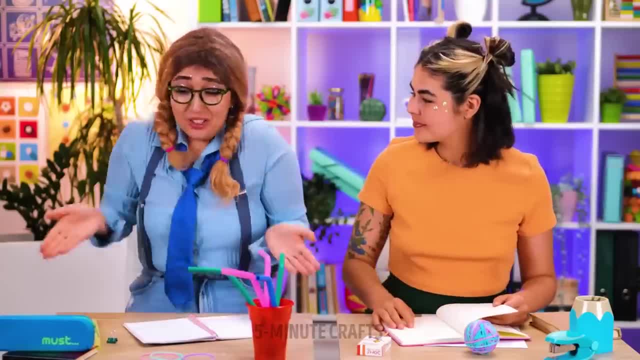 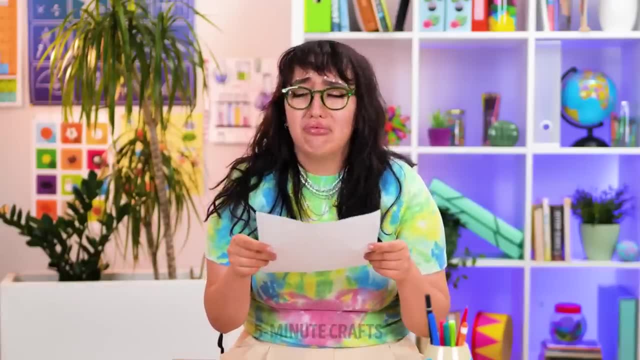 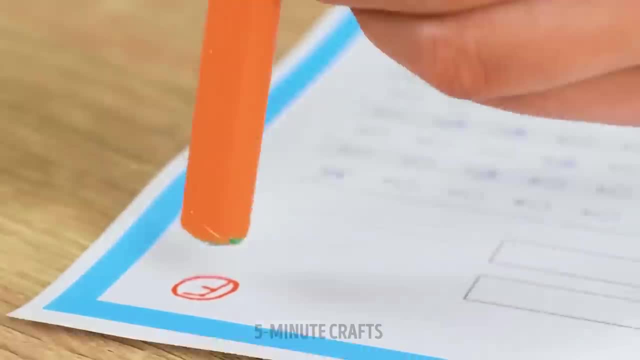 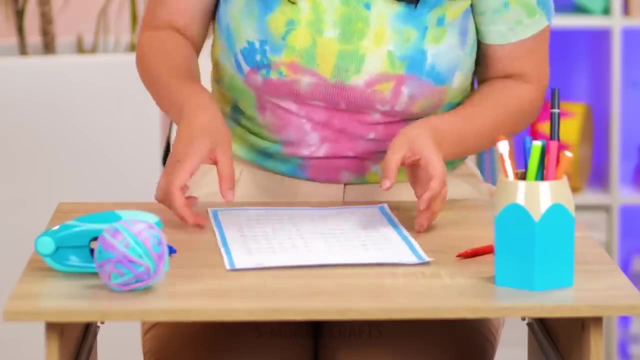 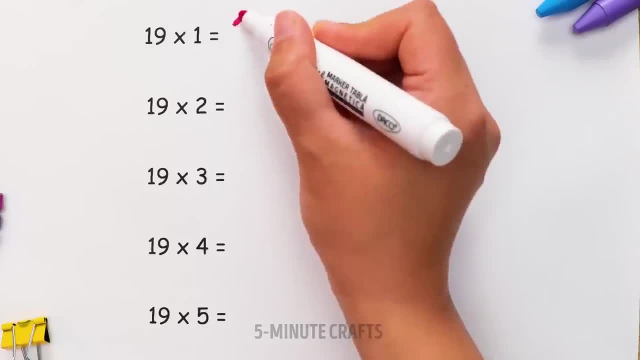 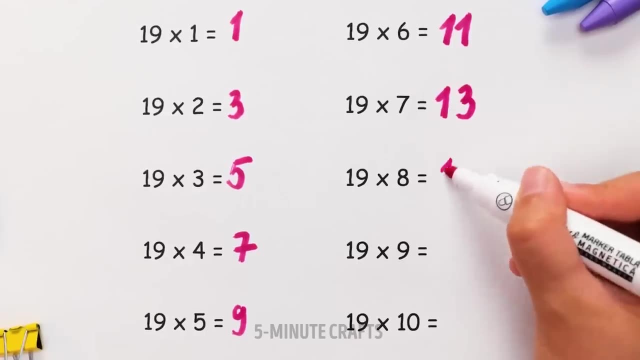 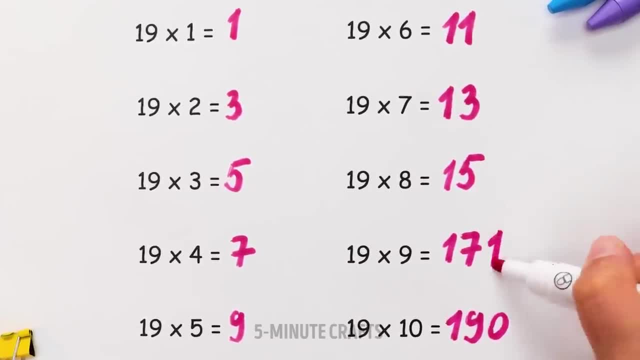 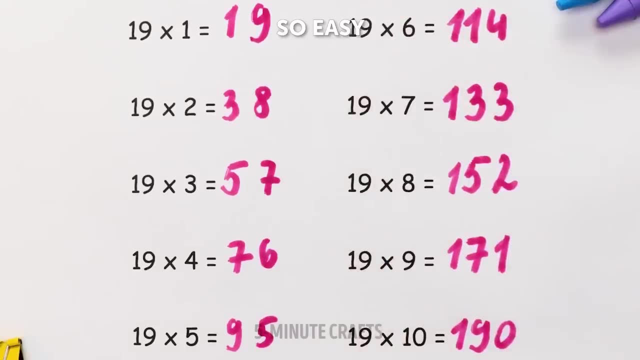 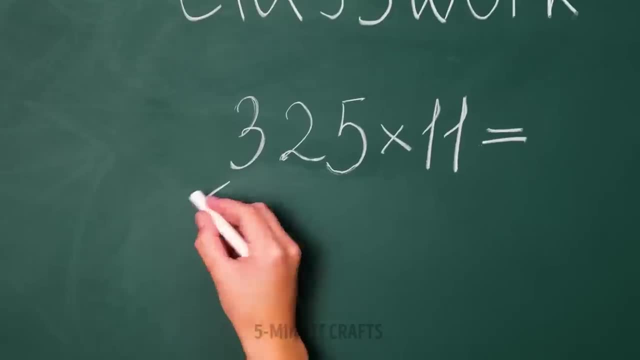 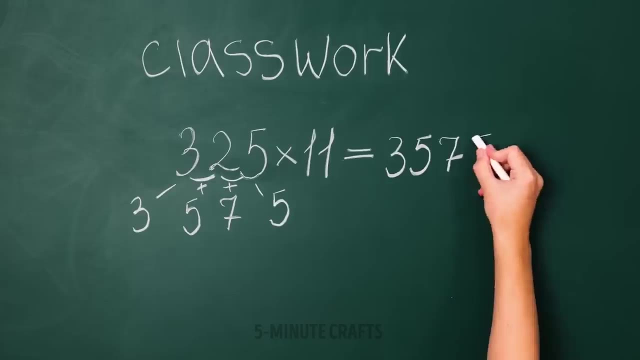 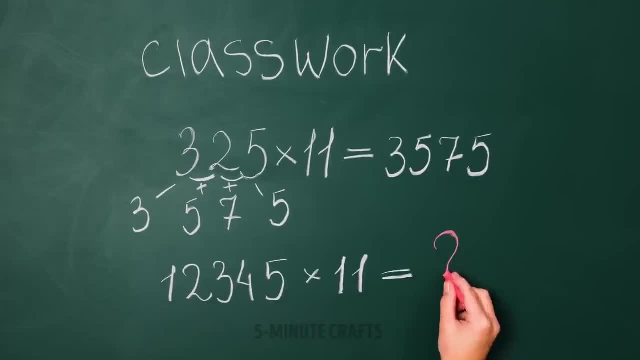 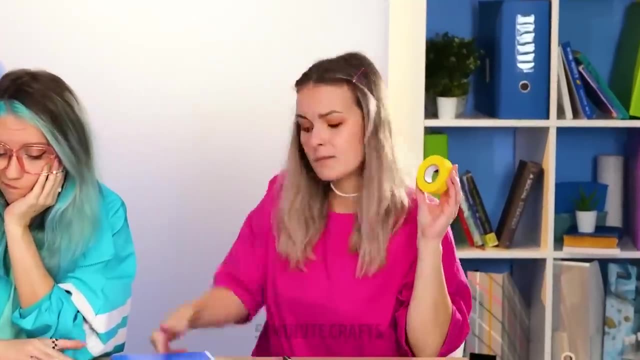 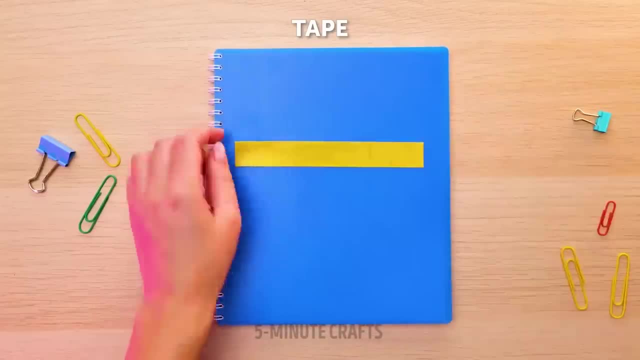 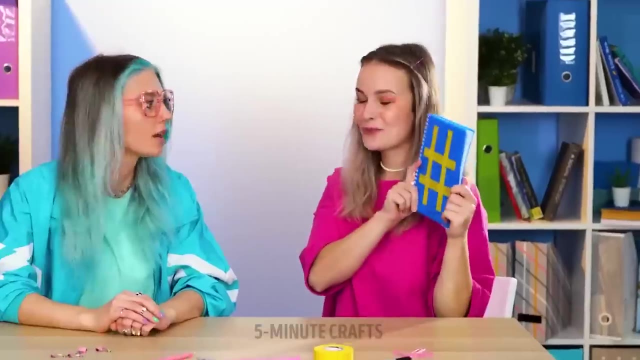 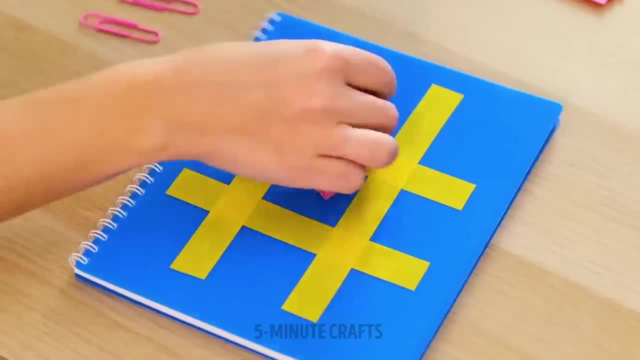 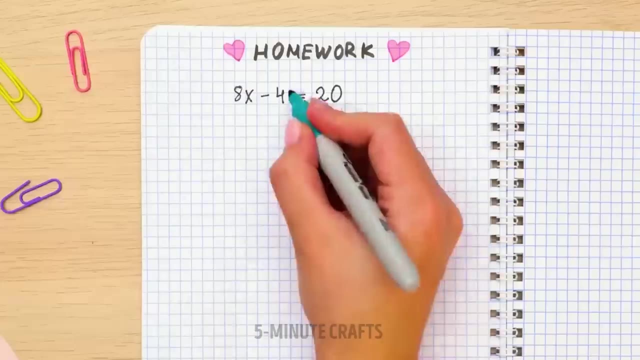 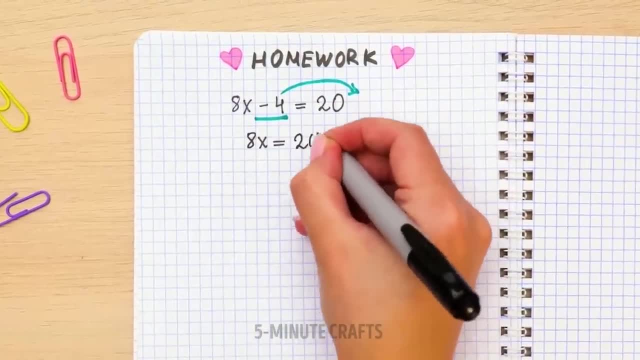 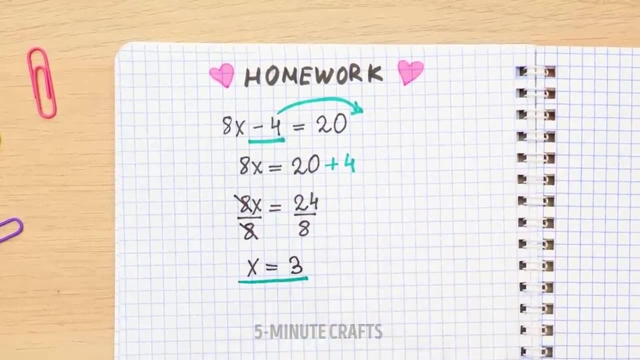 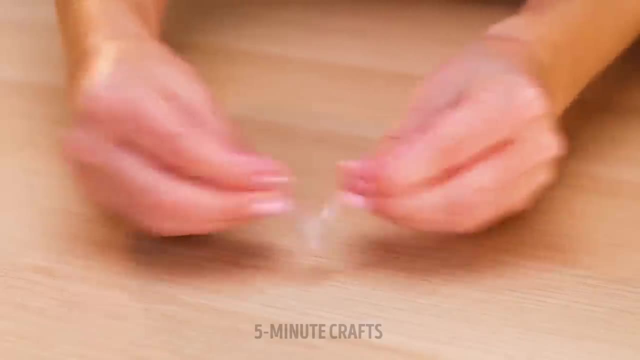 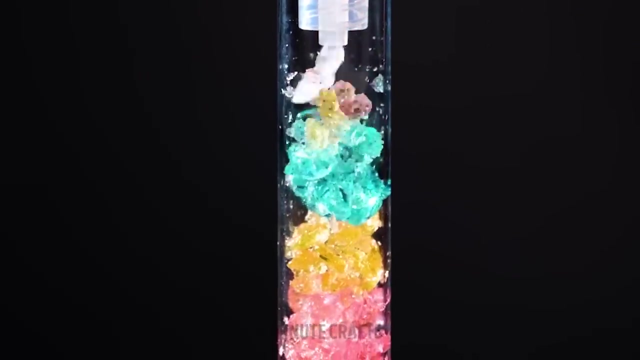 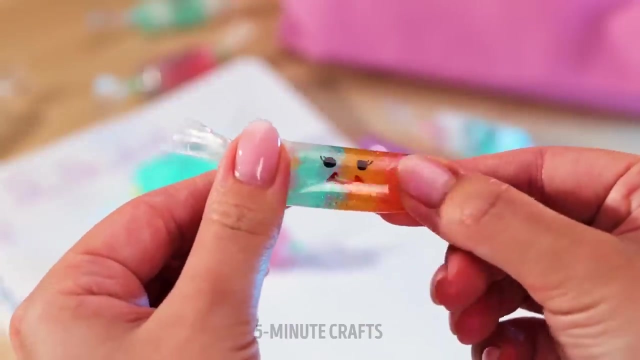 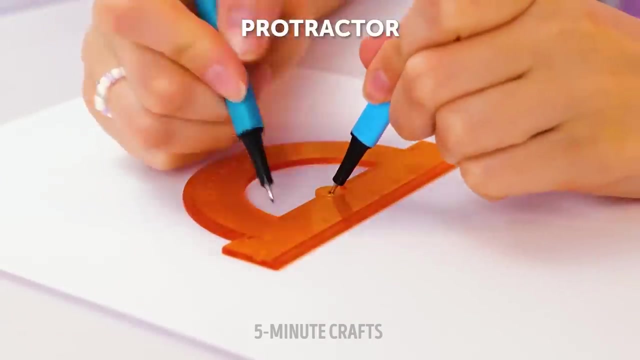 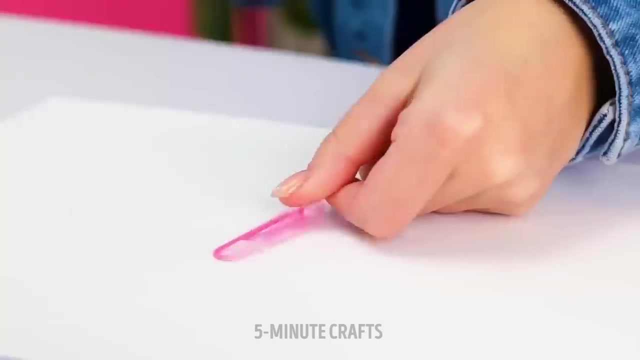 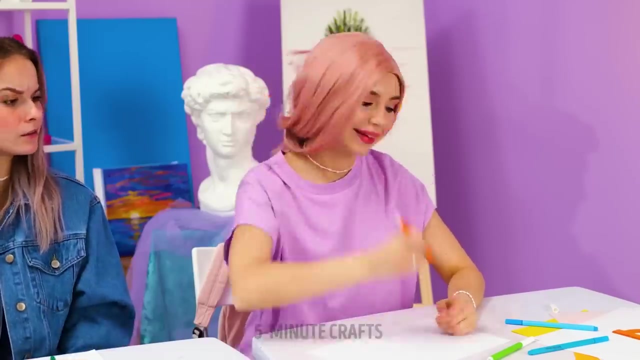 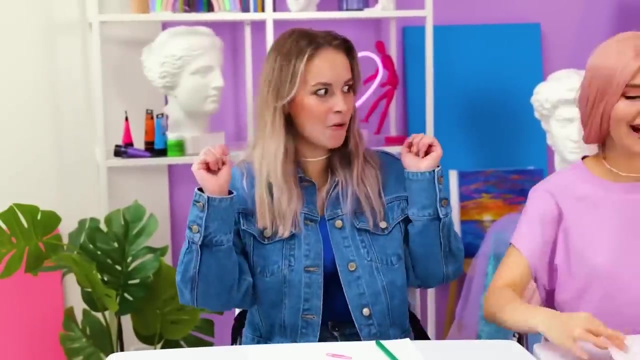 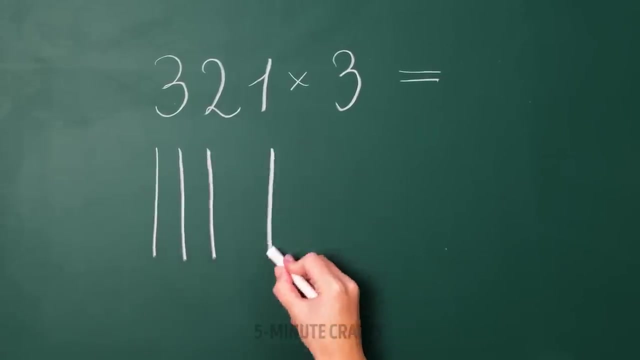 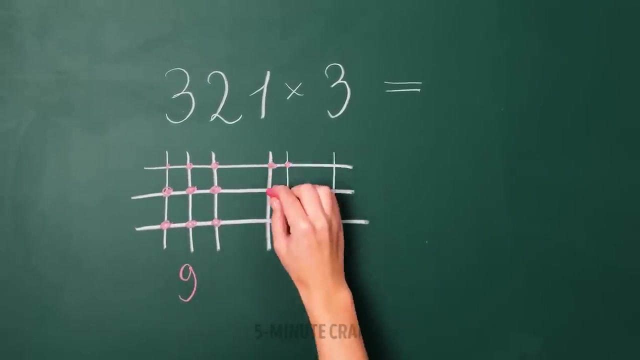 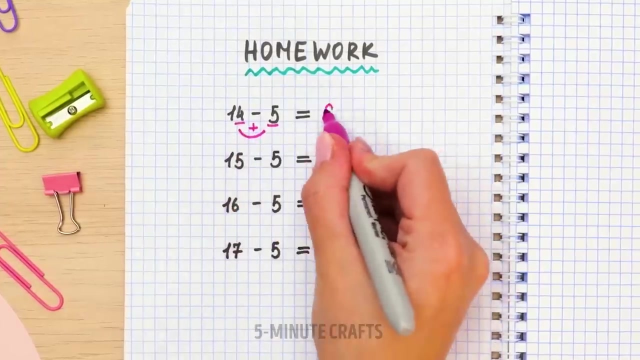 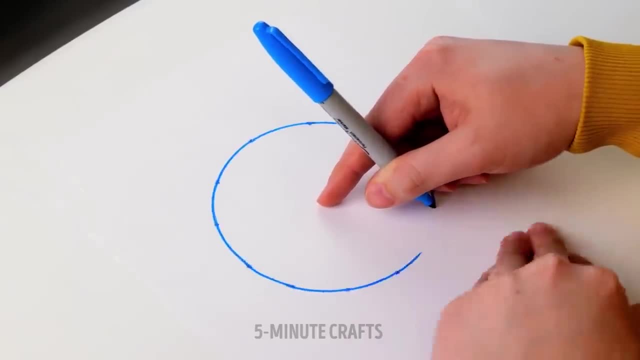 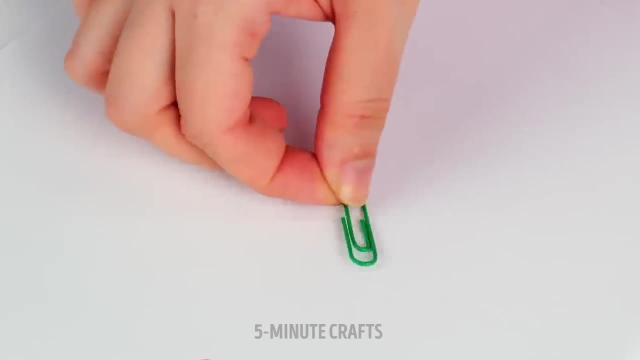 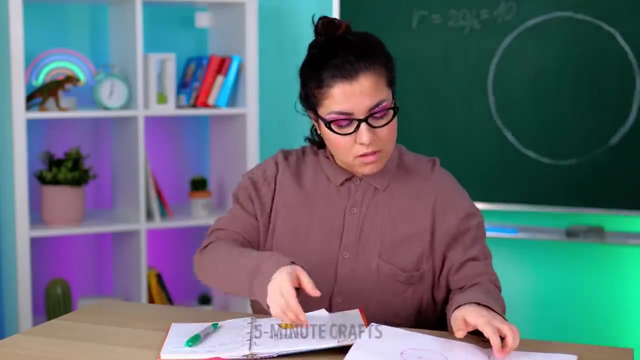 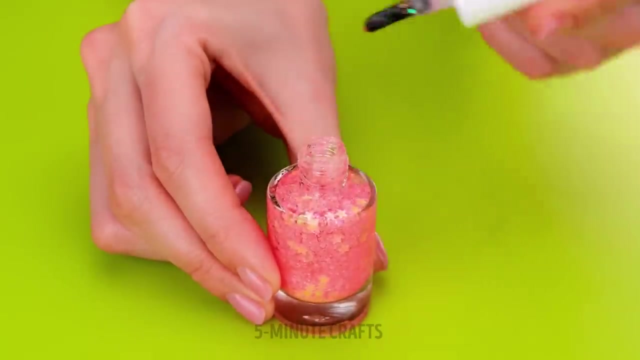 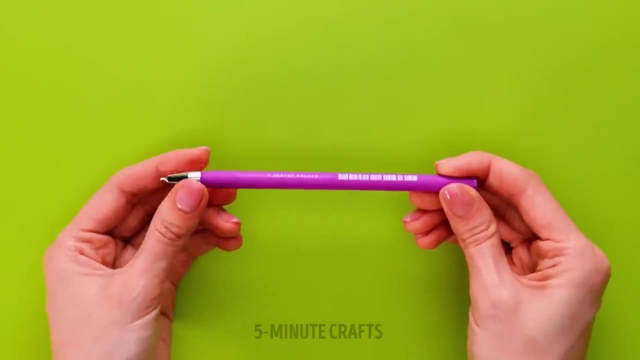 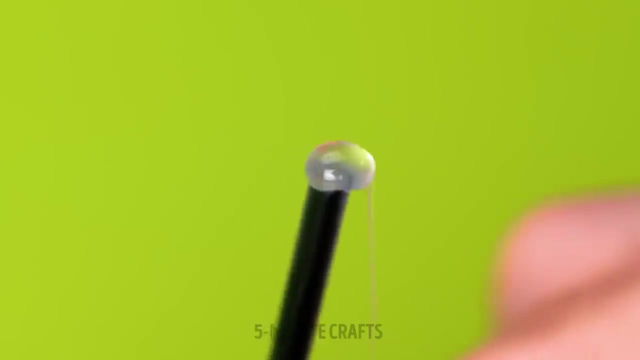 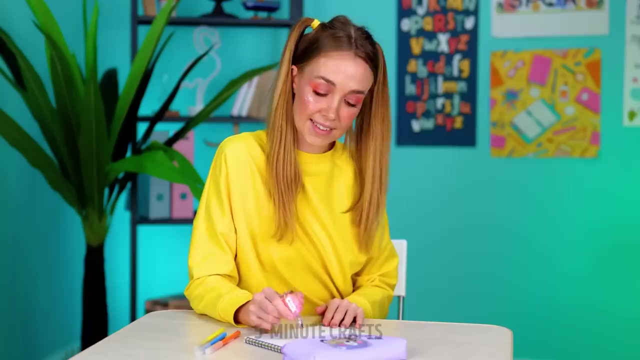 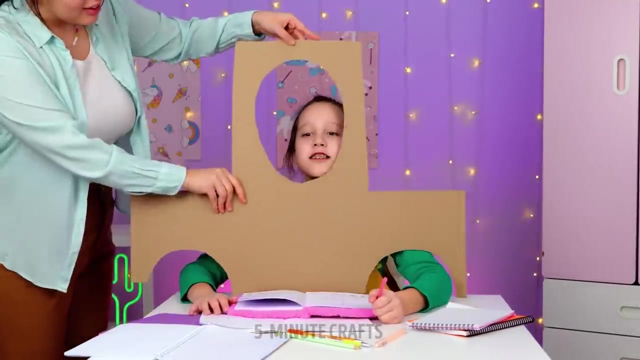 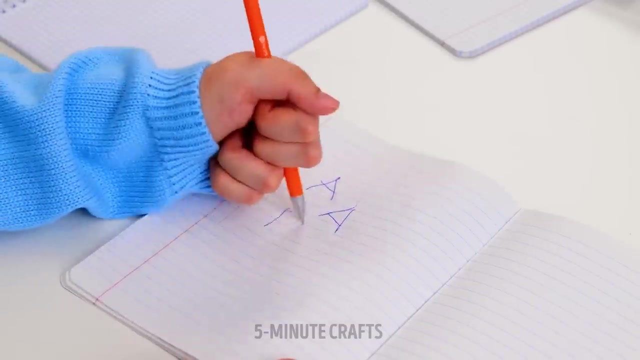 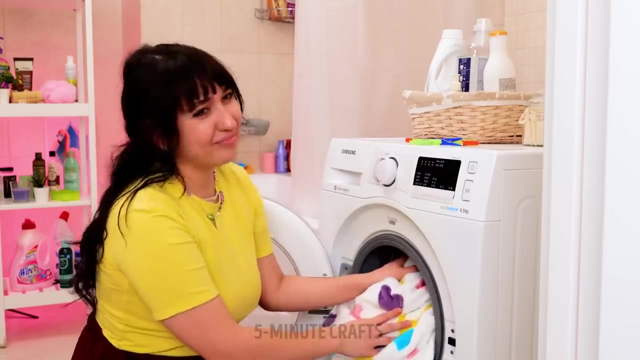 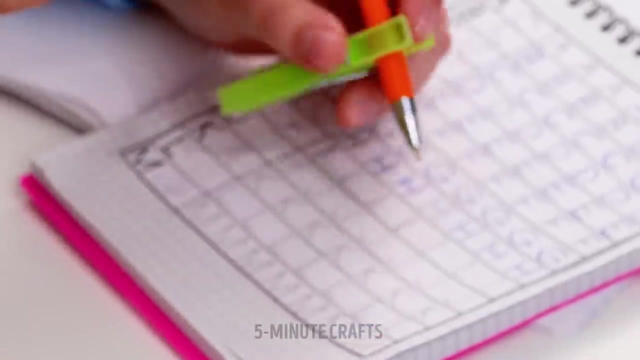 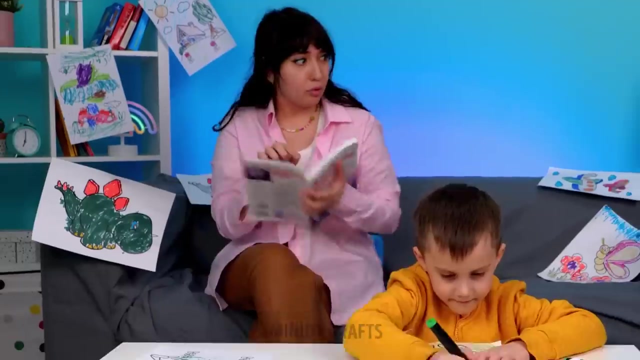 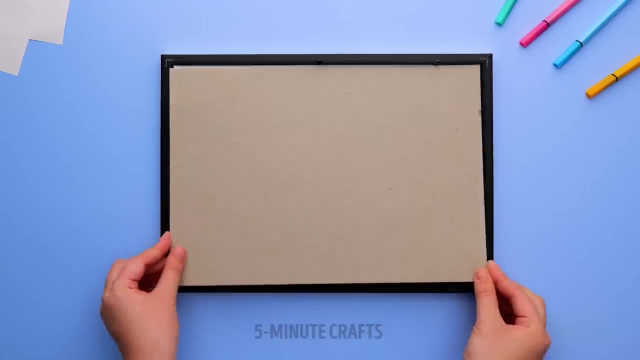 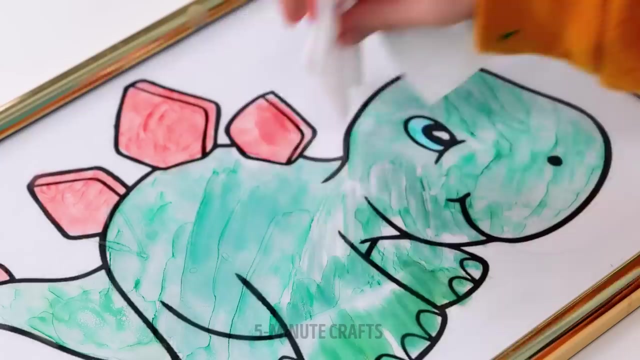 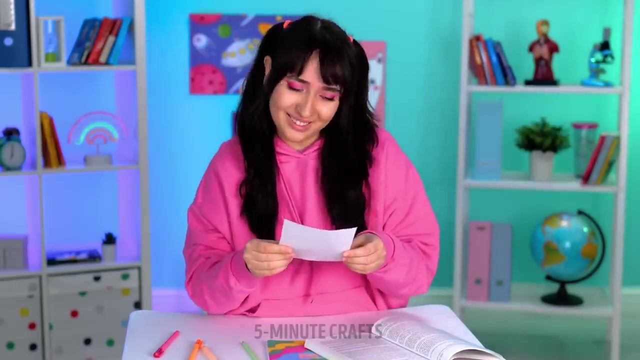 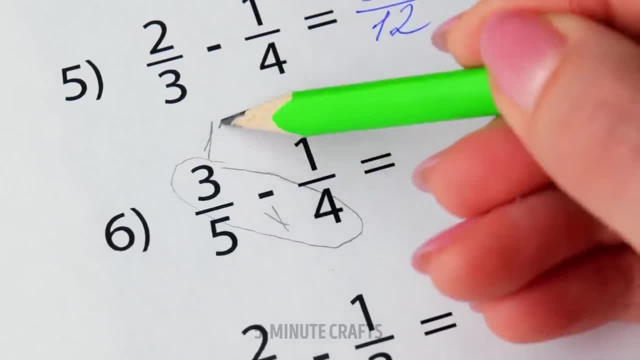 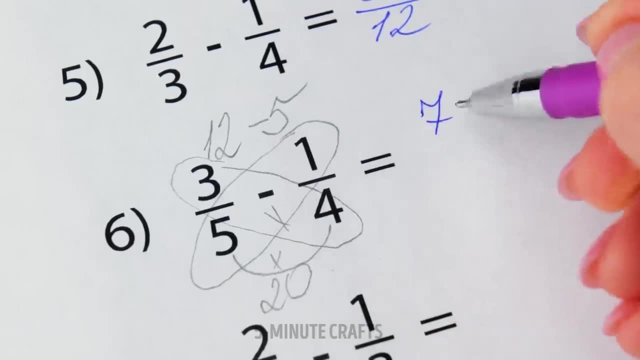 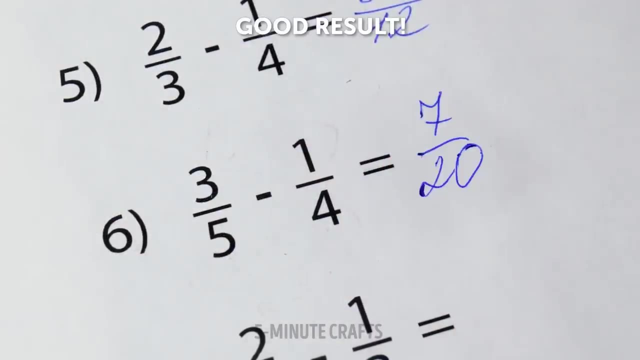 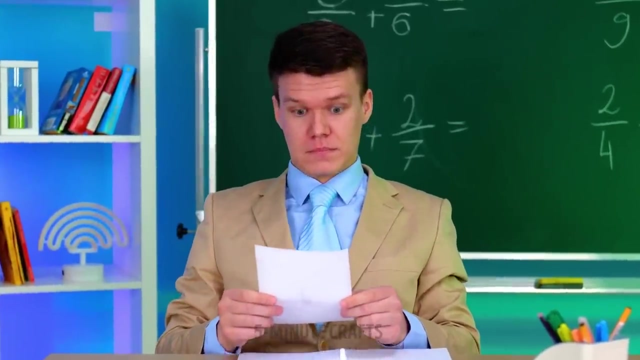 humming. No, my body don't move like that. Don't make me pretend I don't see your shortcomings. You'll be running when I raise the black flag. Get out your bomb and fly away. We'll be dancing with our hands in the air when our new dawn is rising. 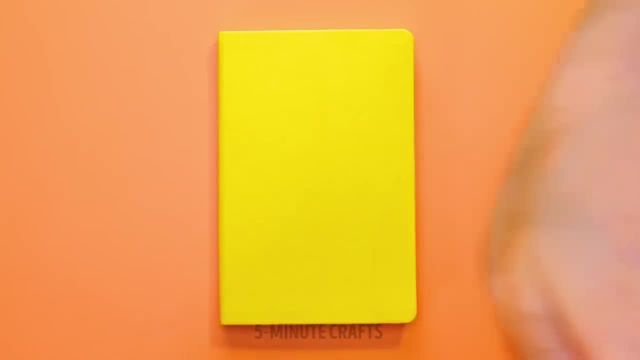 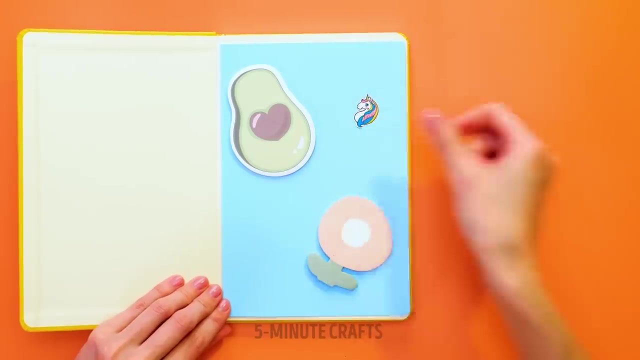 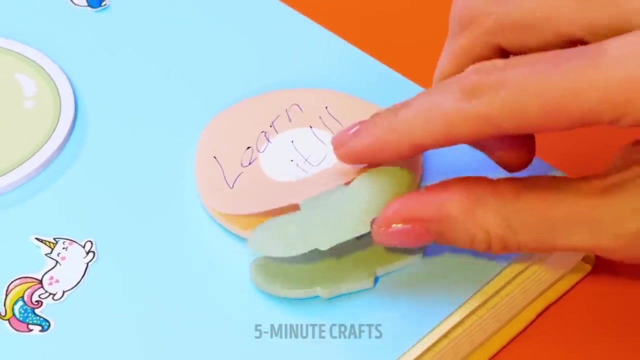 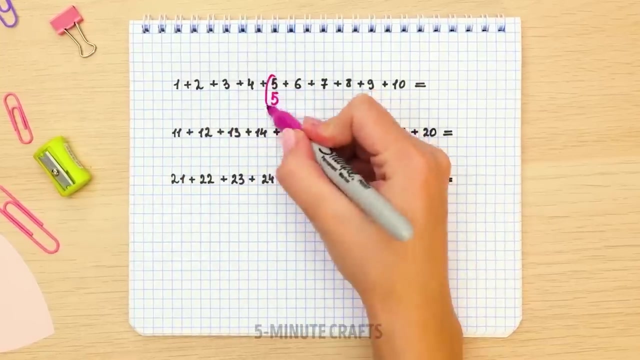 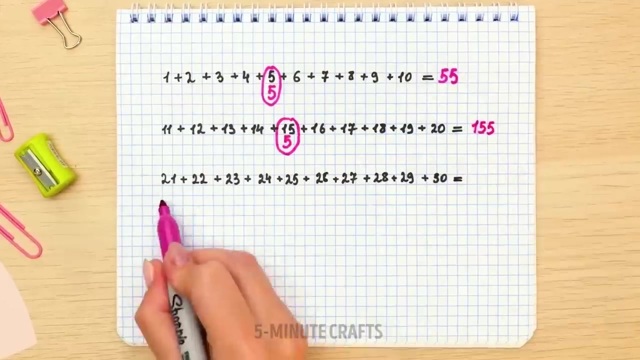 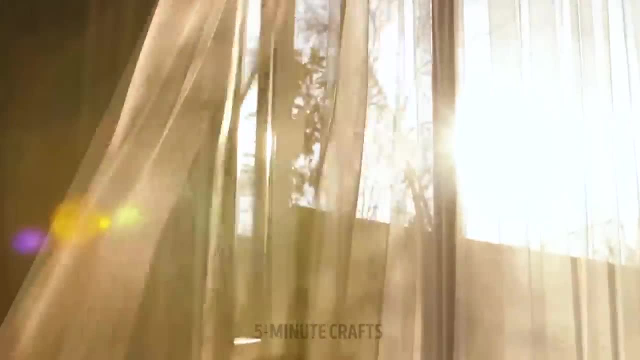 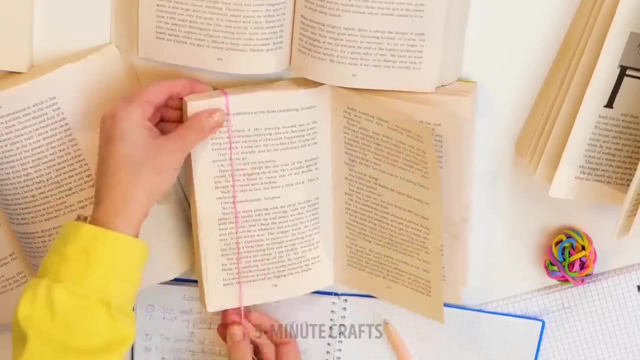 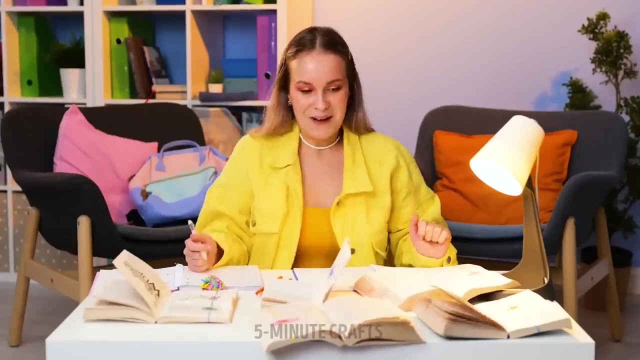 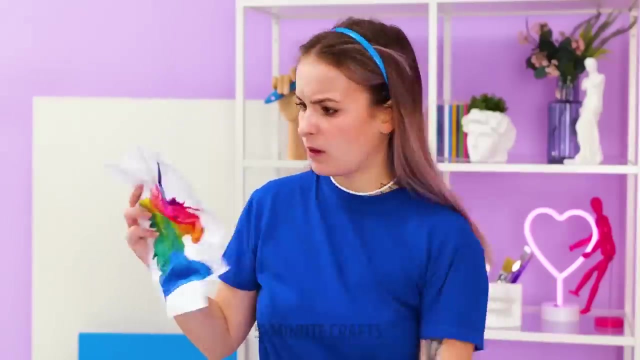 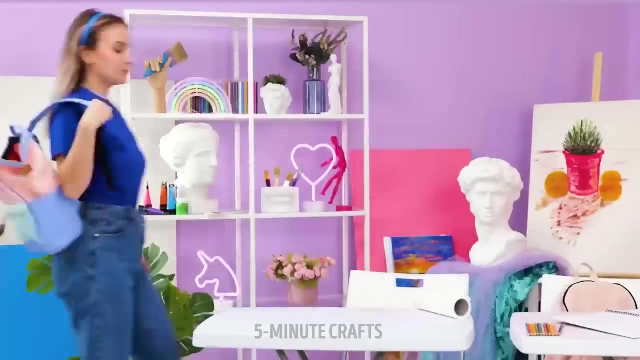 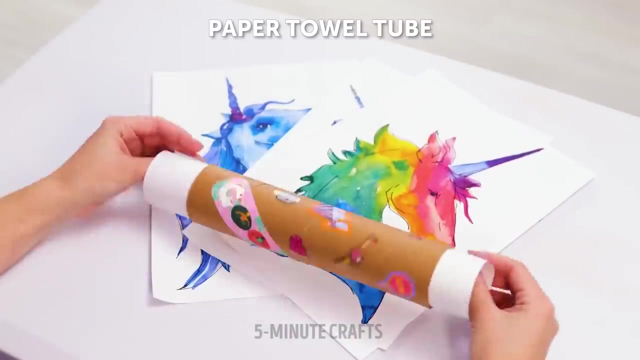 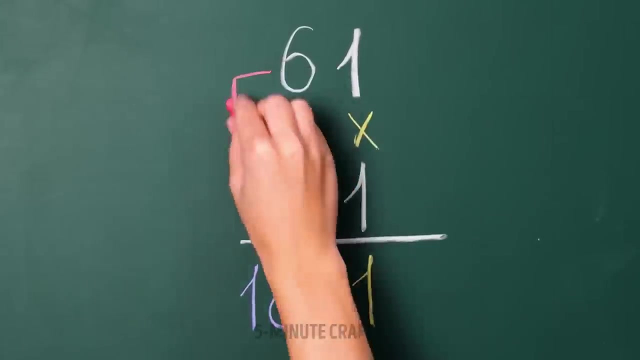 Get out your bomb and fly away. We'll be dancing With our heads in the air When our new dawn is rising. We'll be dancing With our heads in the air When our new dawn is rising. Dancing, We'll be dancing, We'll be dancing, We'll be dancing. 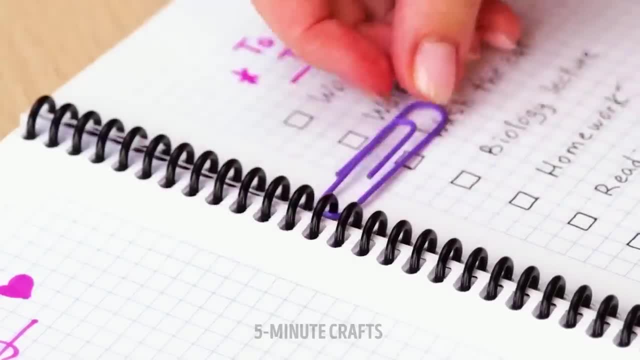 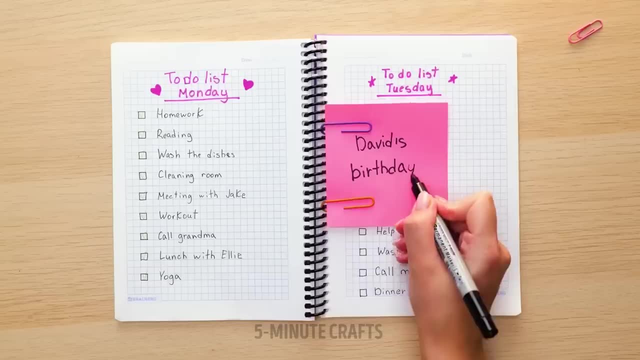 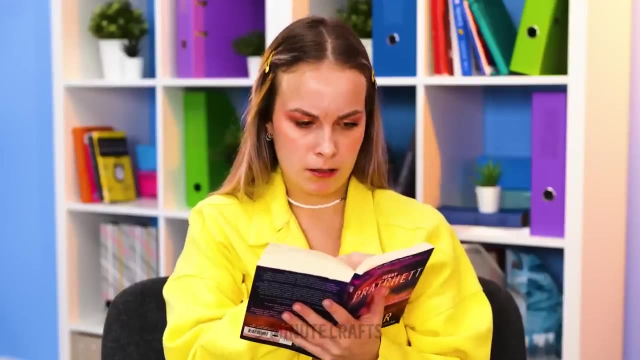 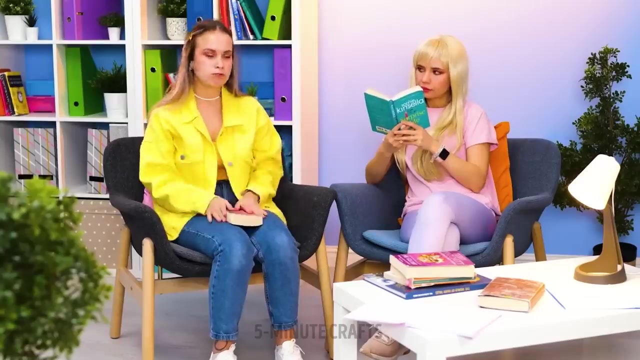 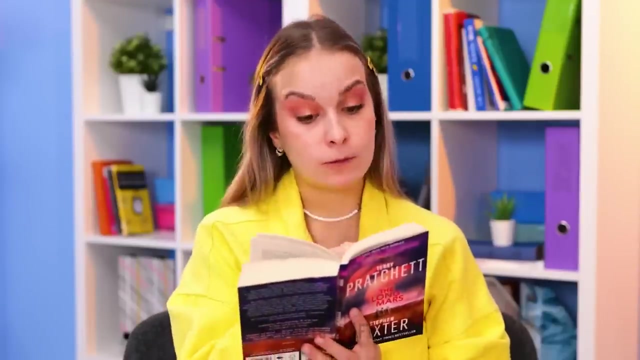 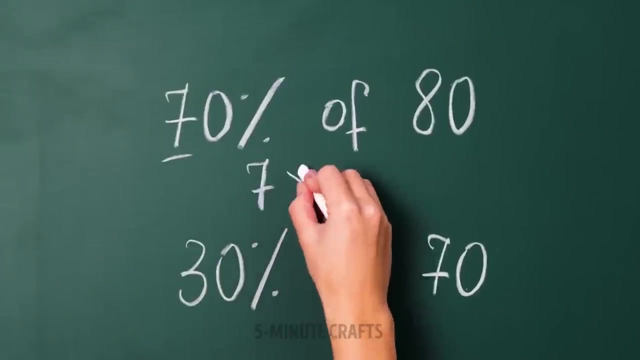 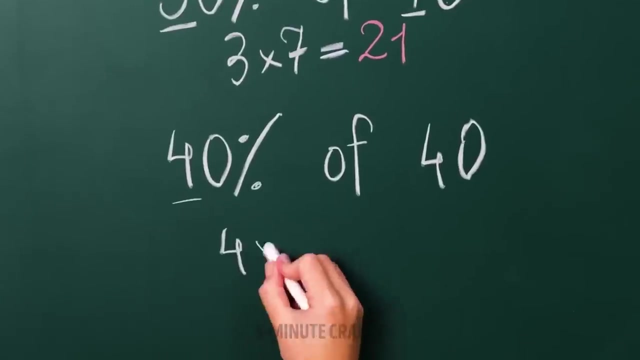 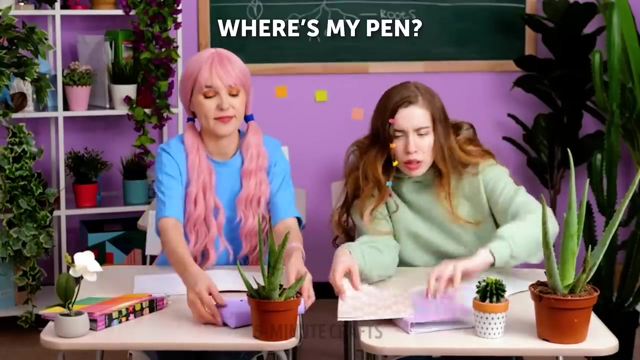 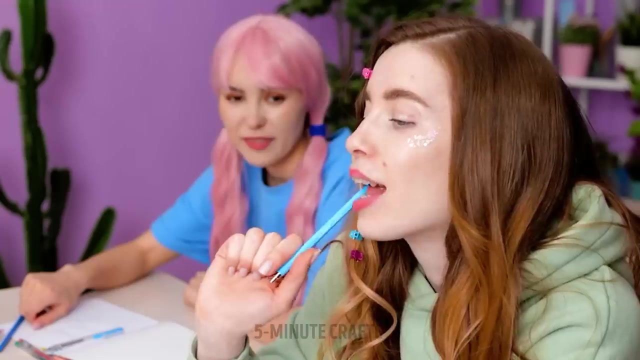 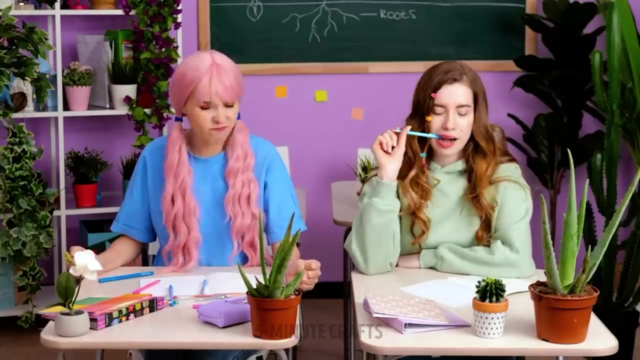 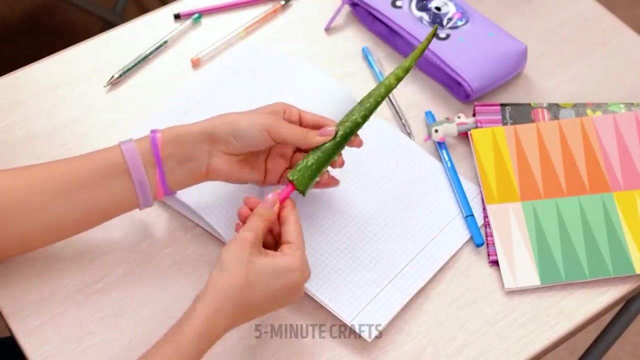 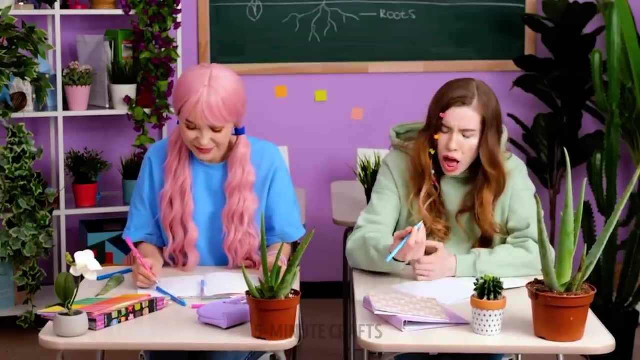 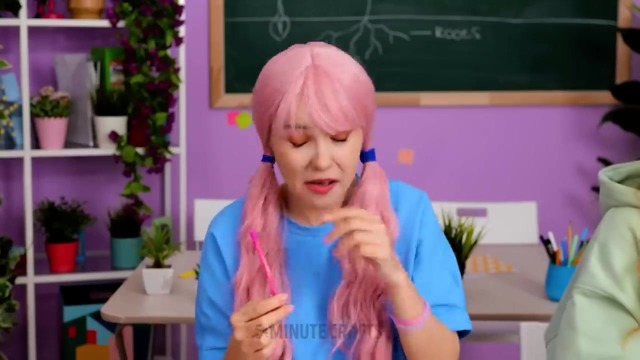 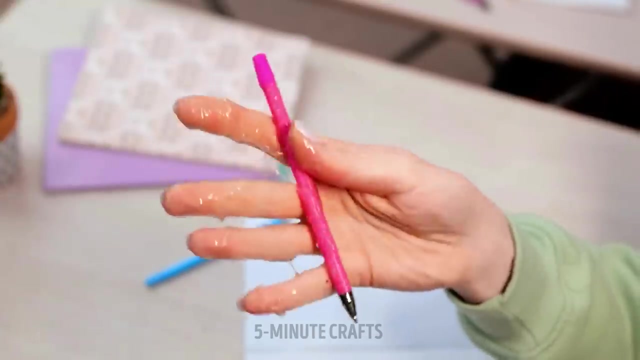 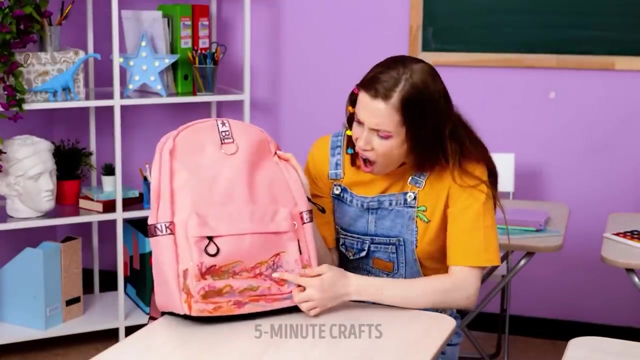 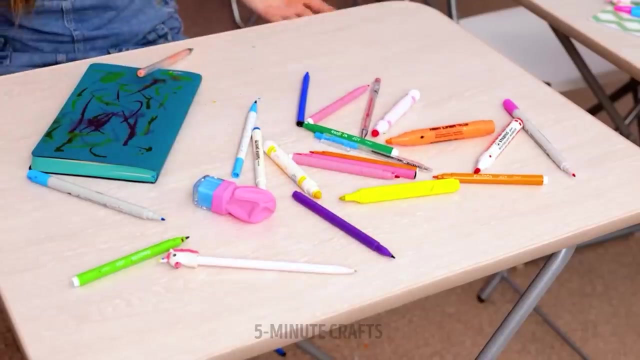 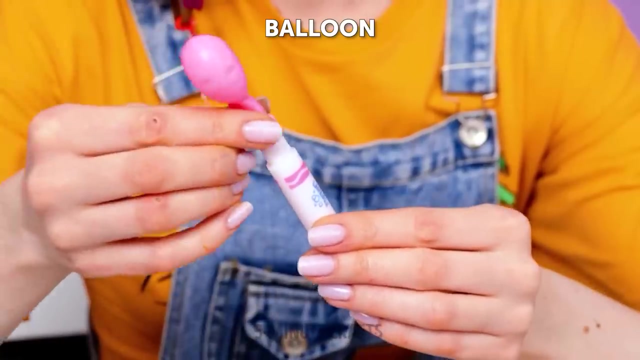 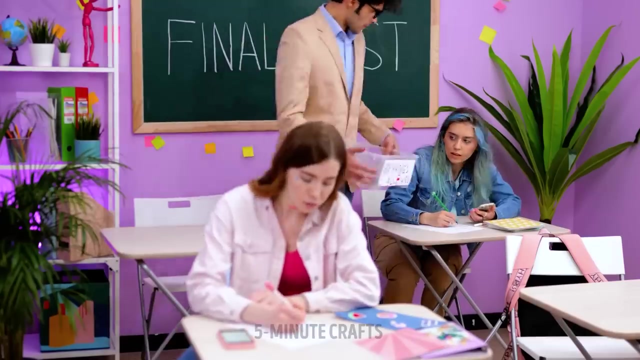 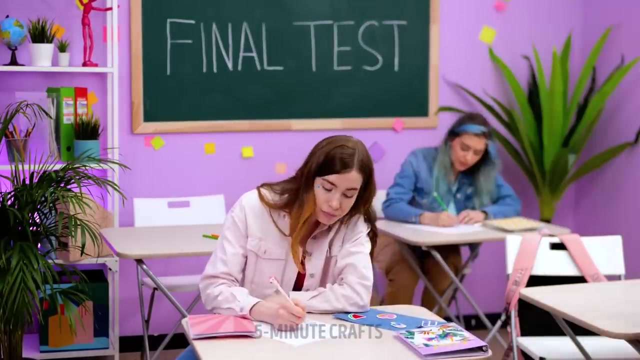 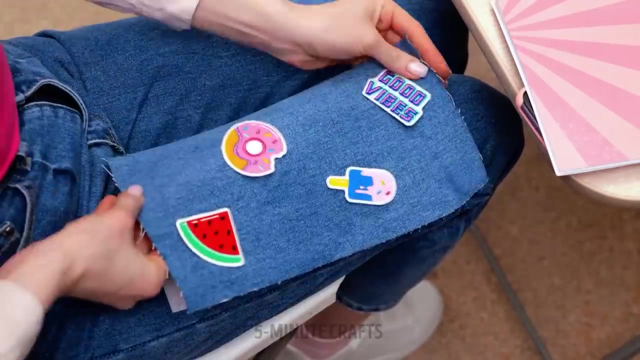 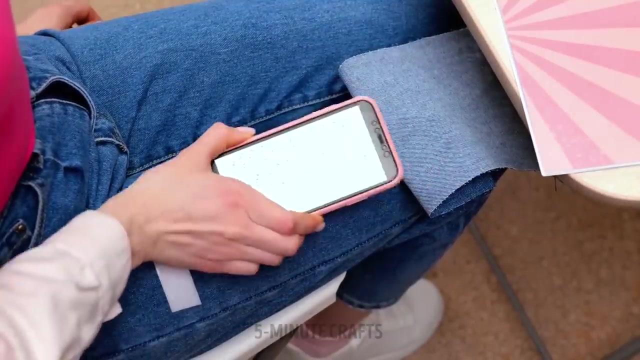 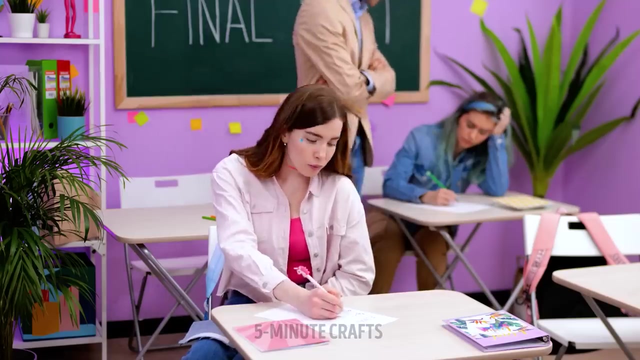 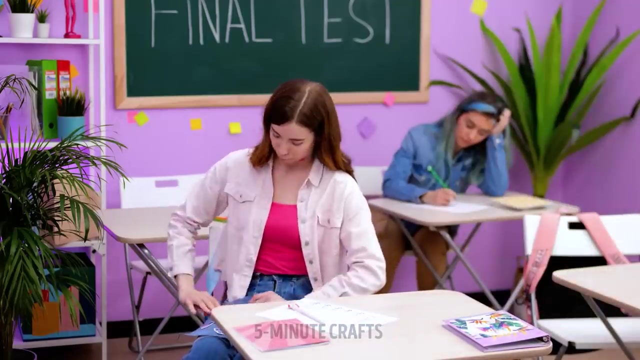 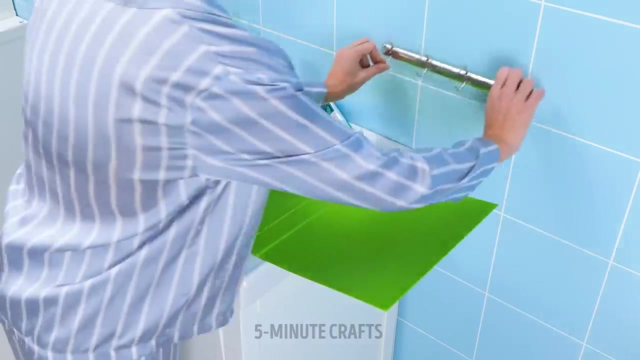 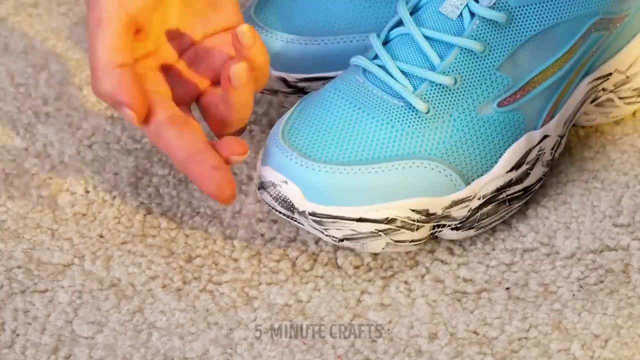 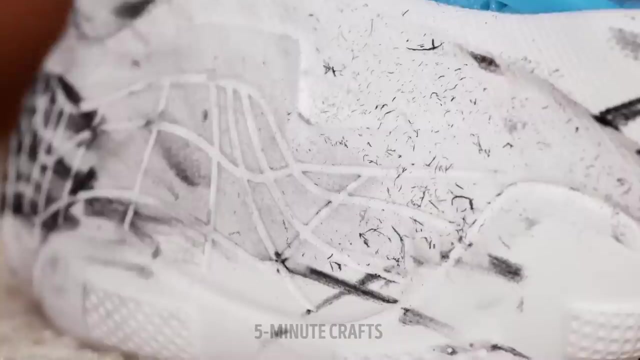 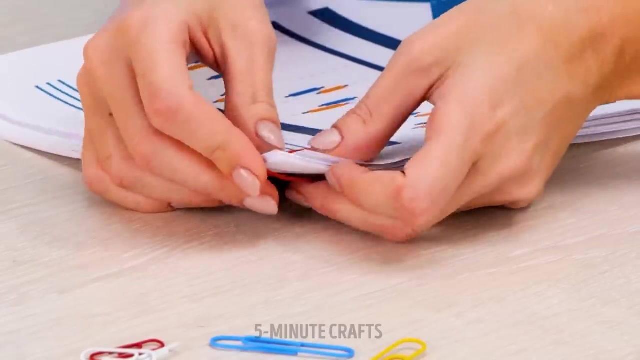 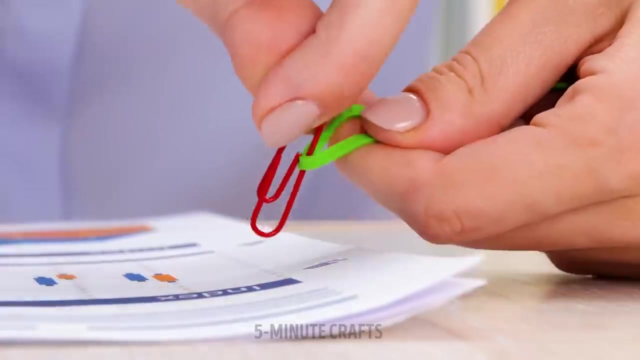 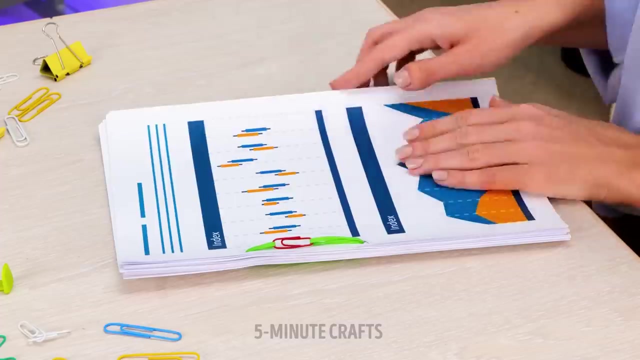 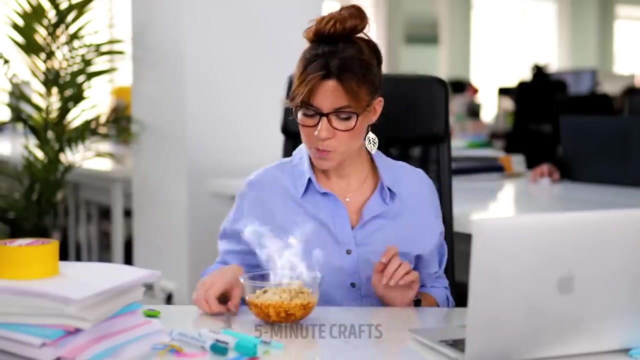 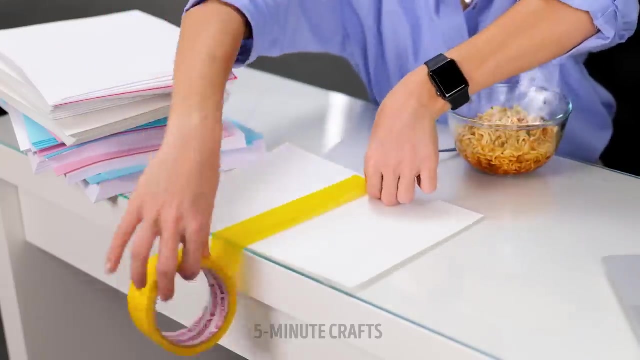 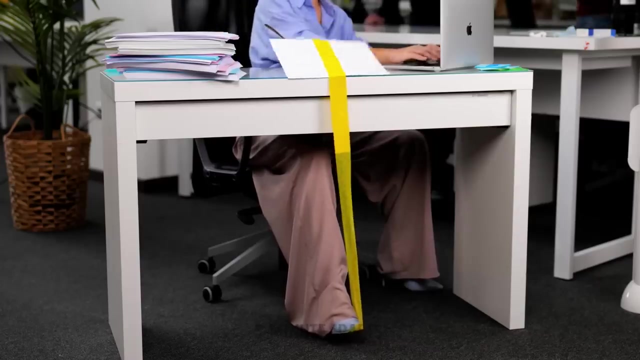 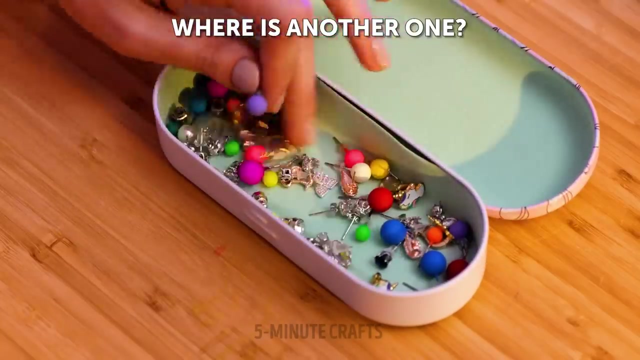 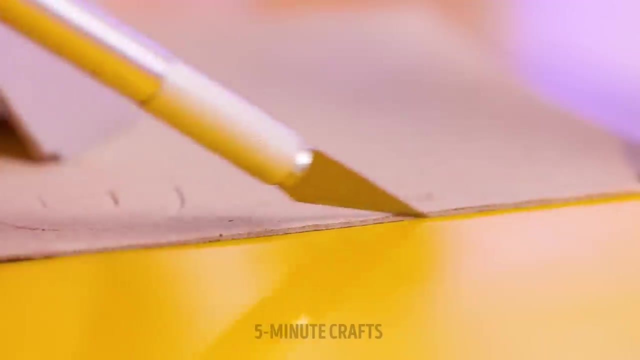 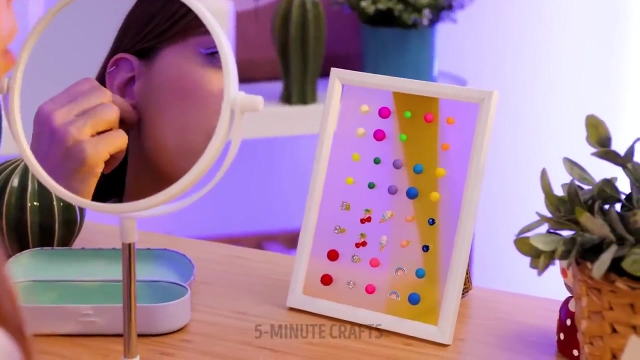 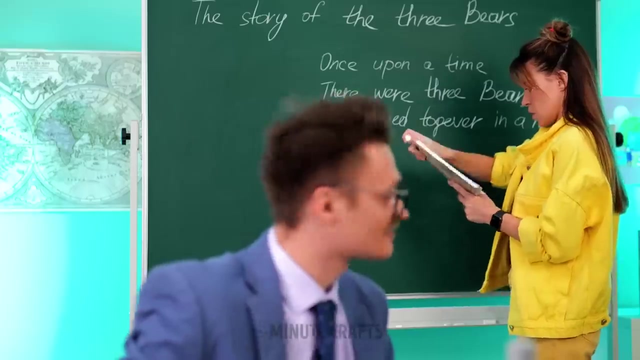 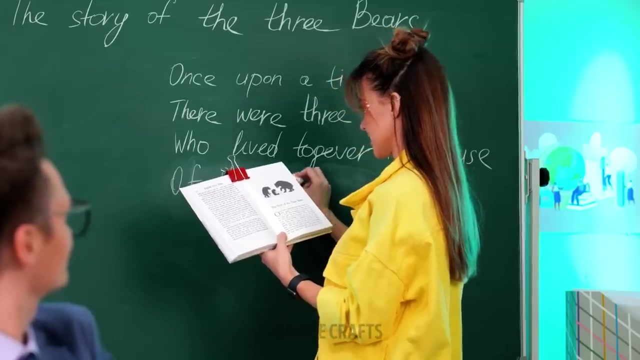 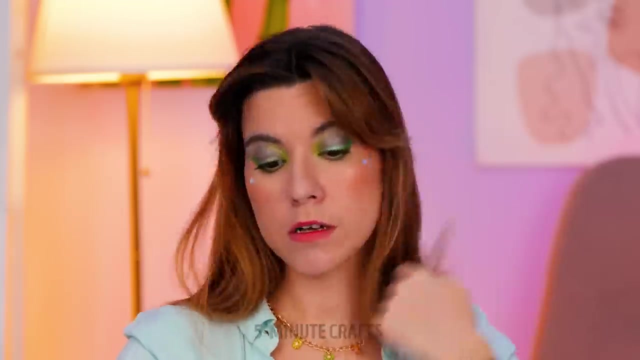 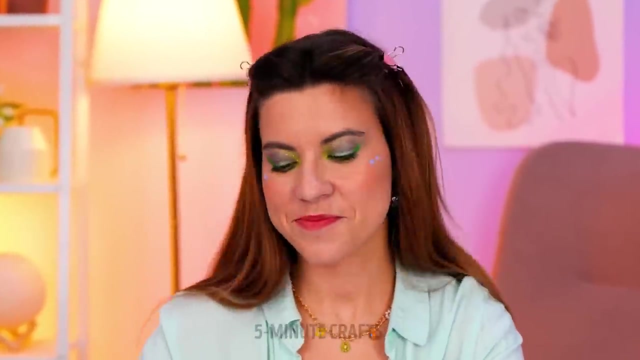 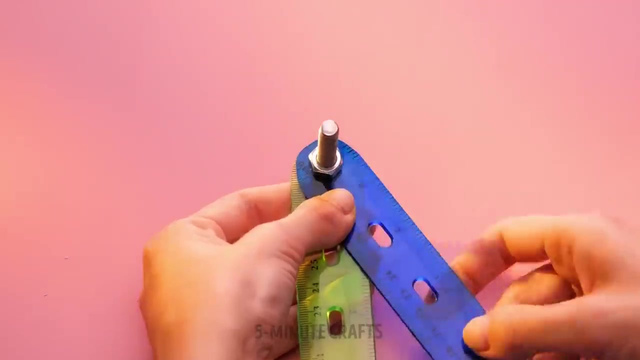 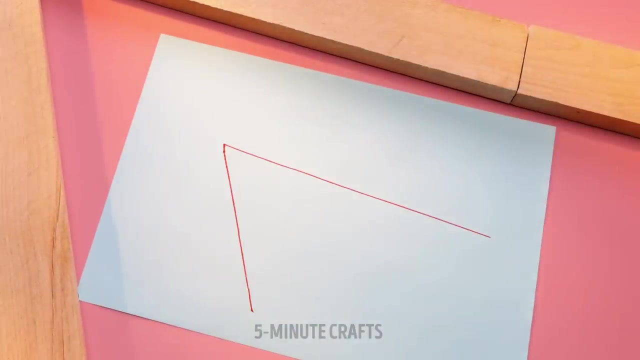 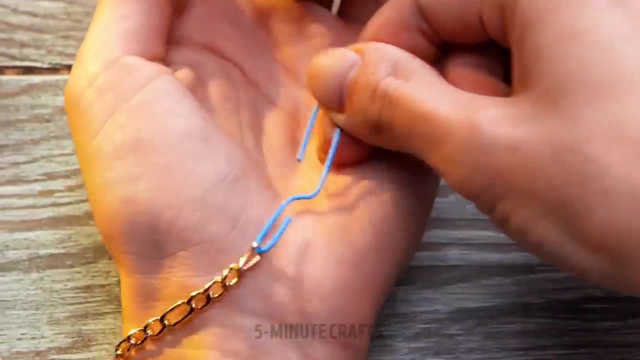 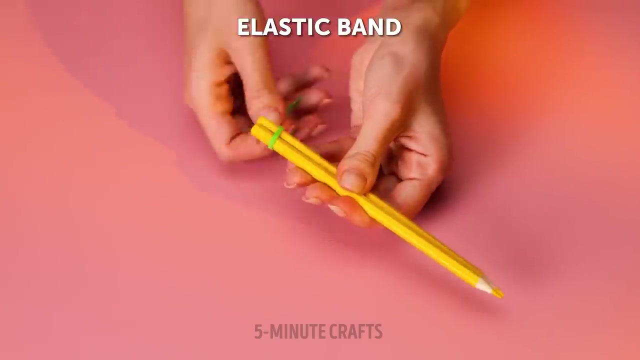 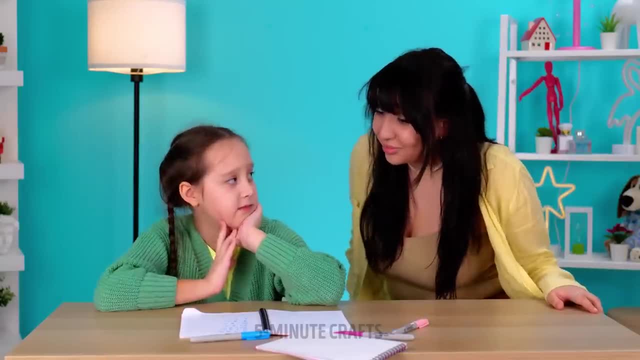 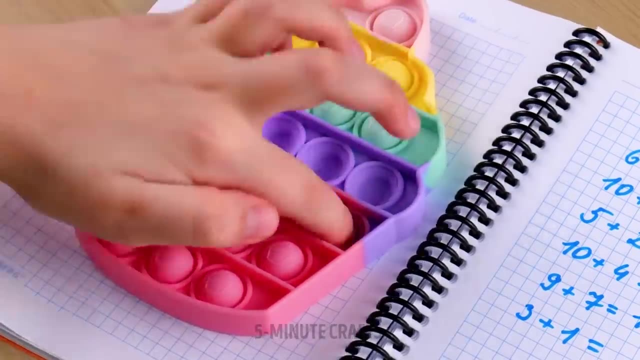 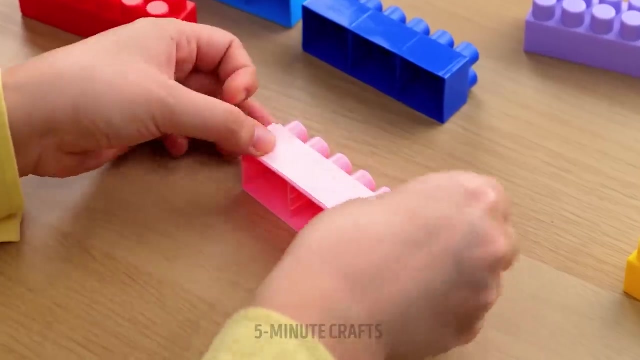 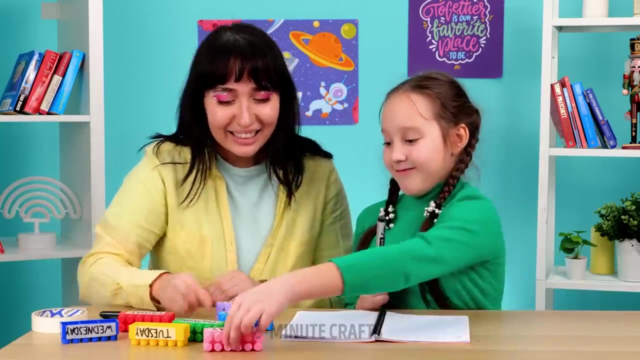 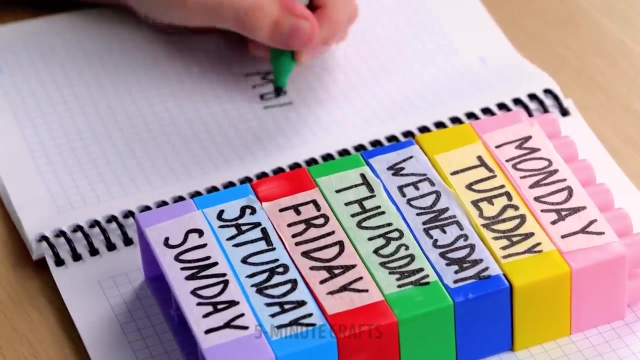 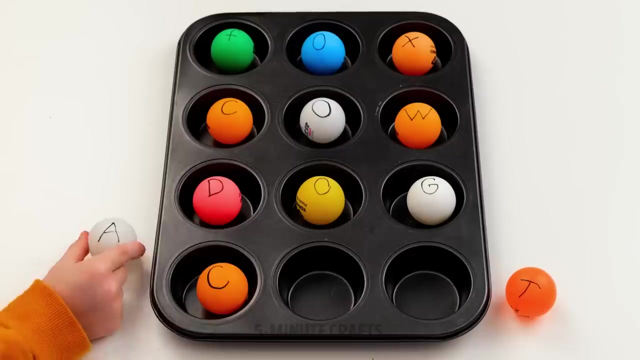 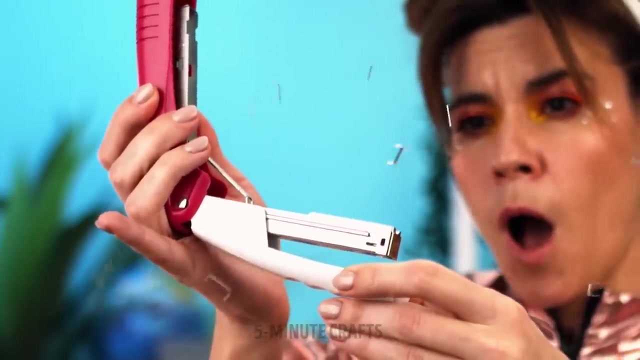 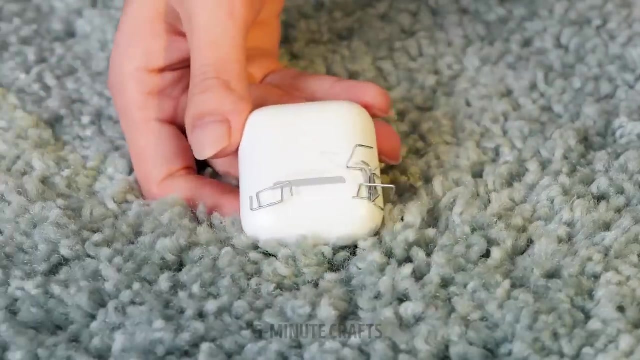 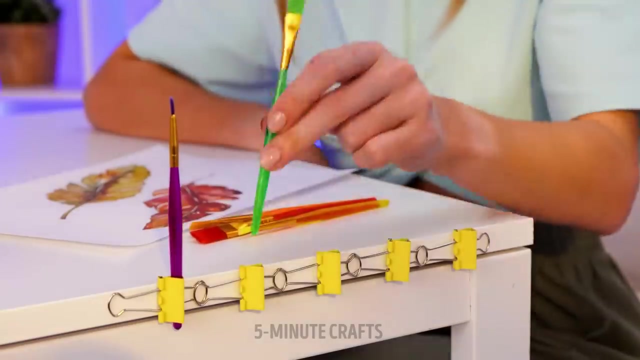 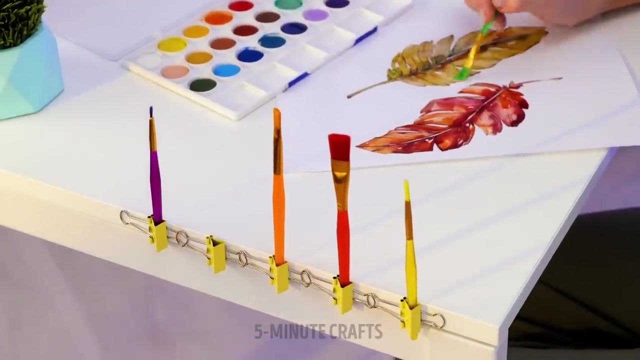 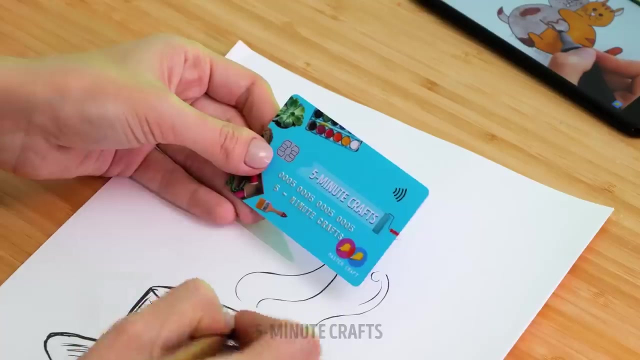 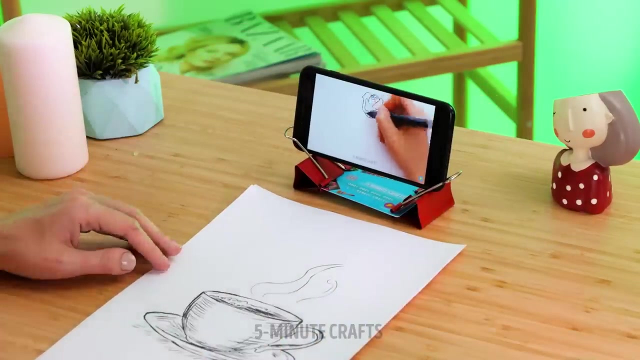 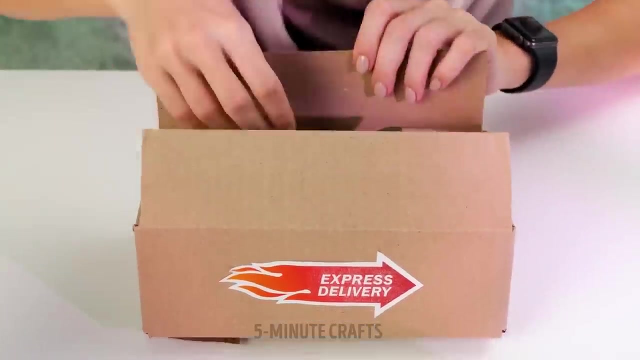 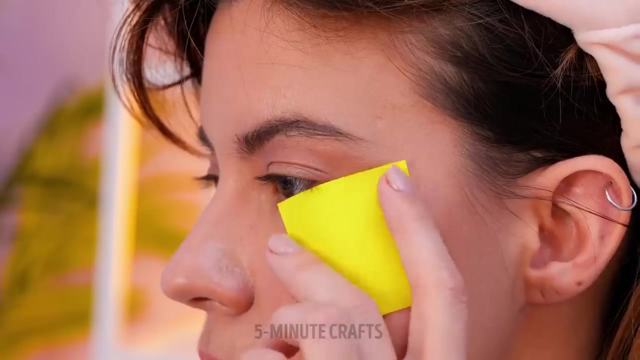 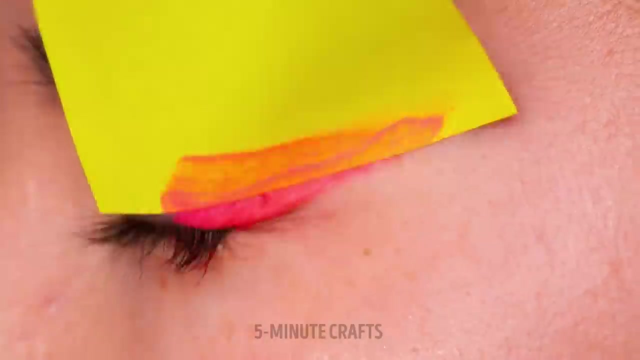 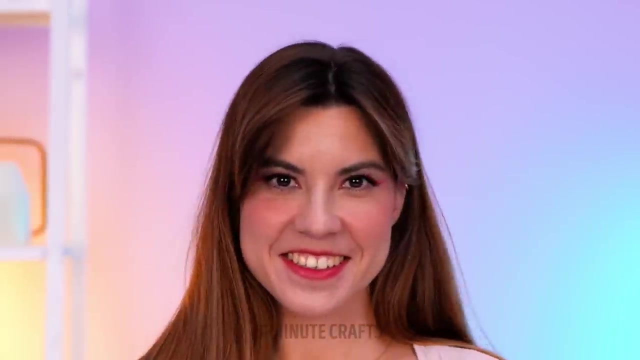 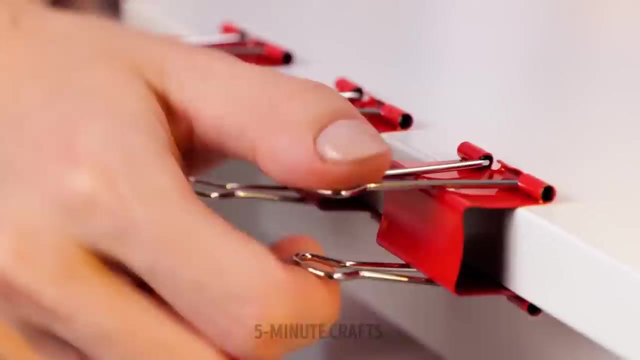 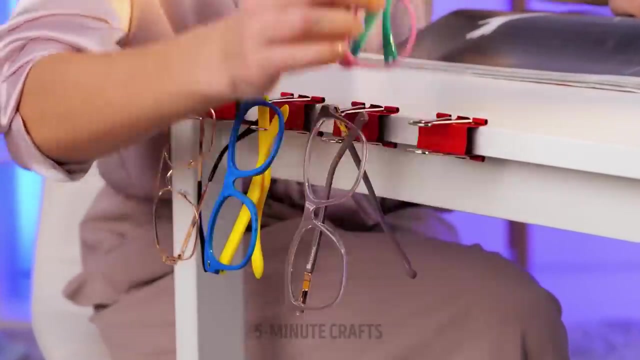 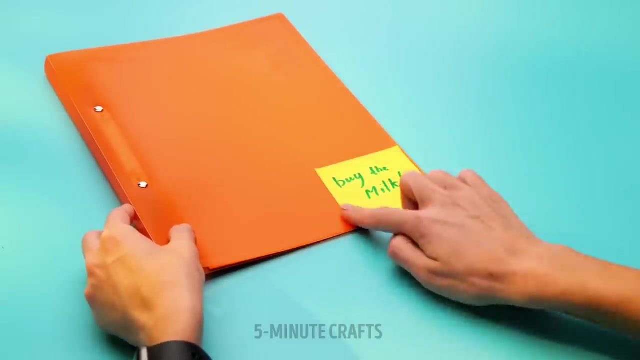 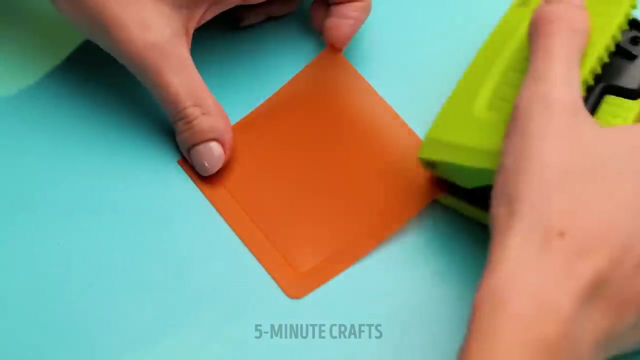 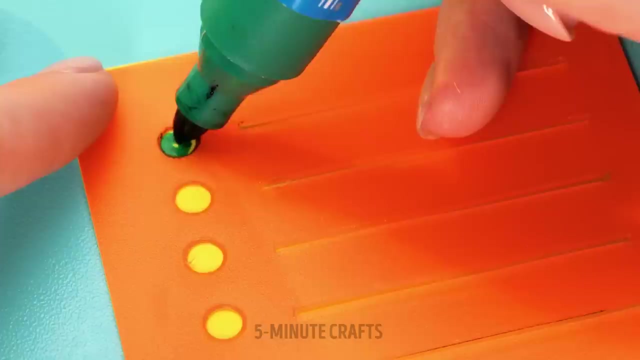 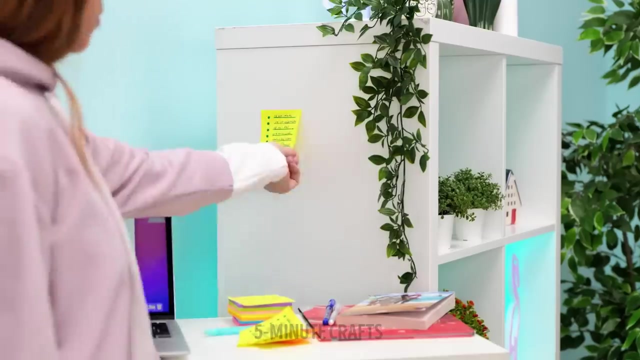 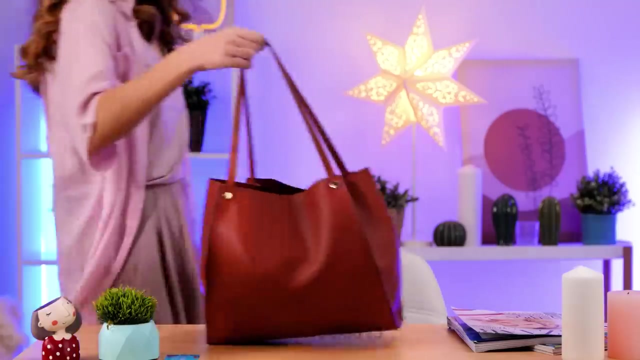 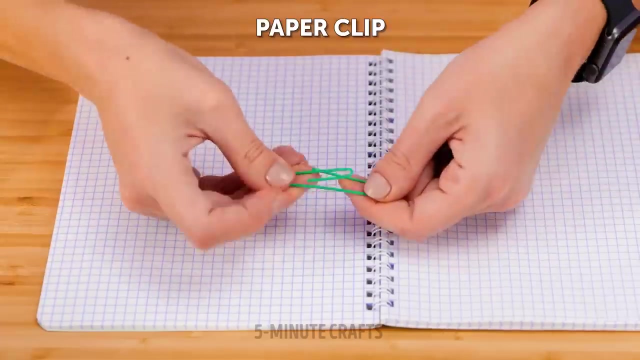 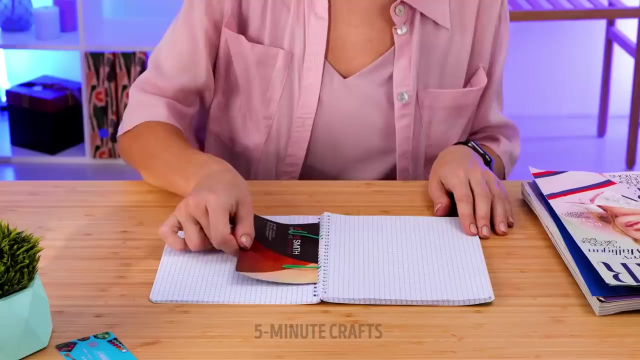 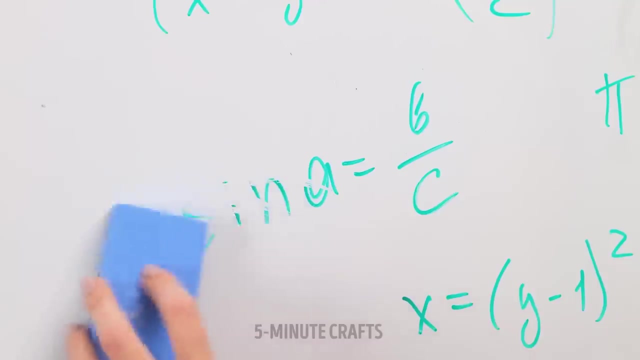 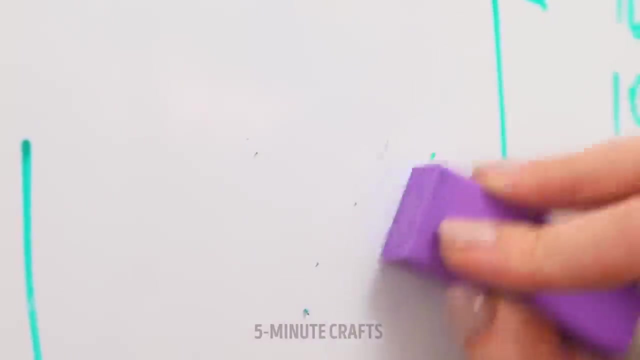 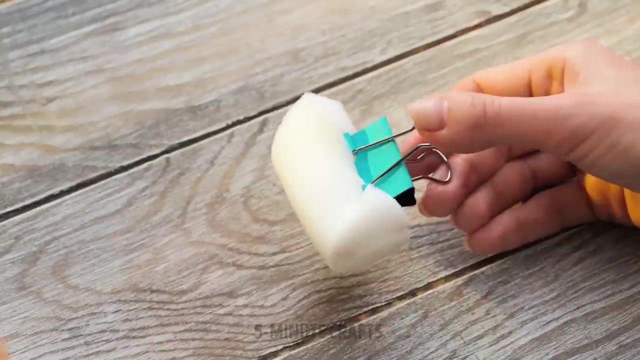 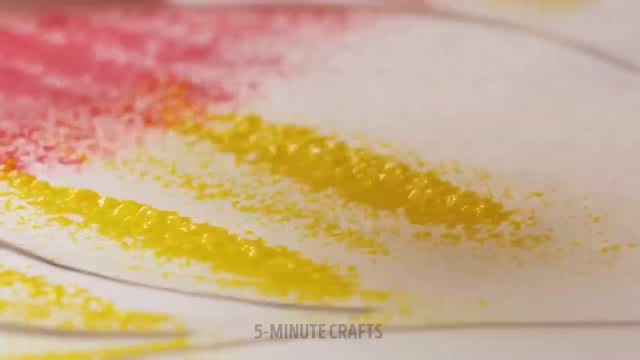 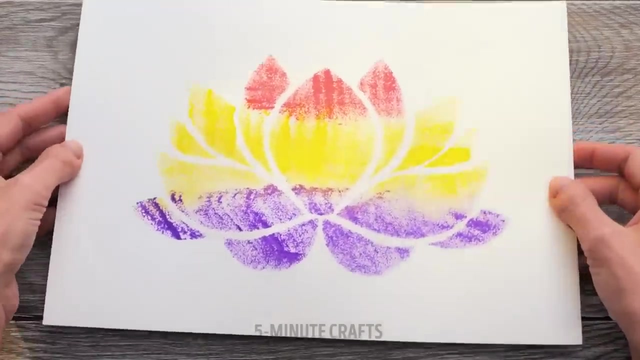 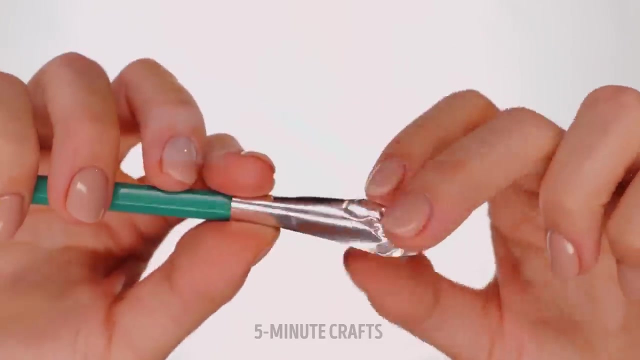 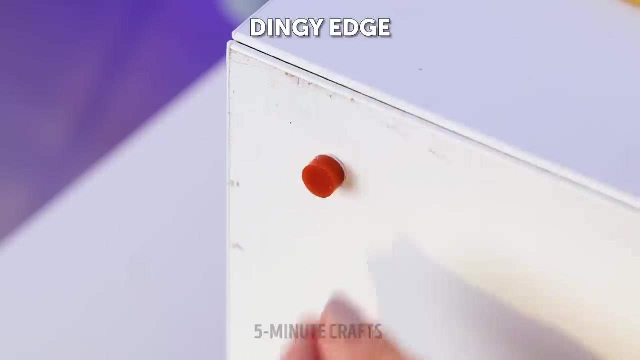 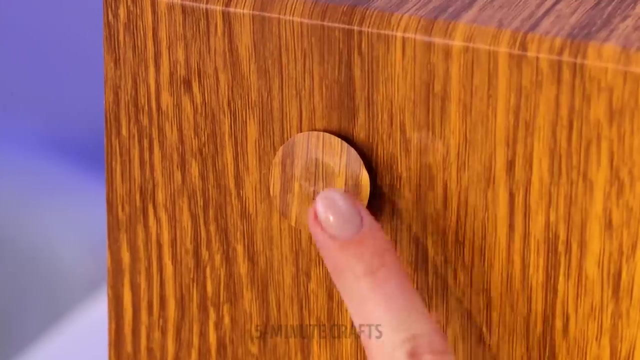 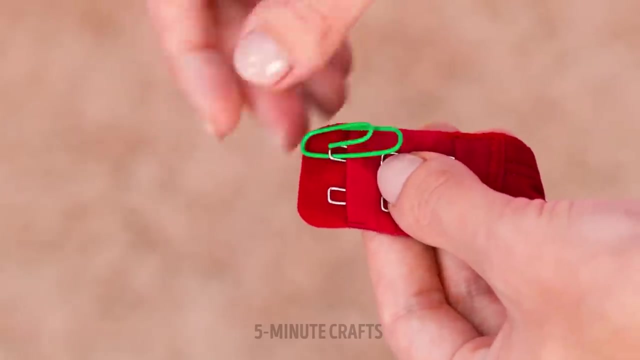 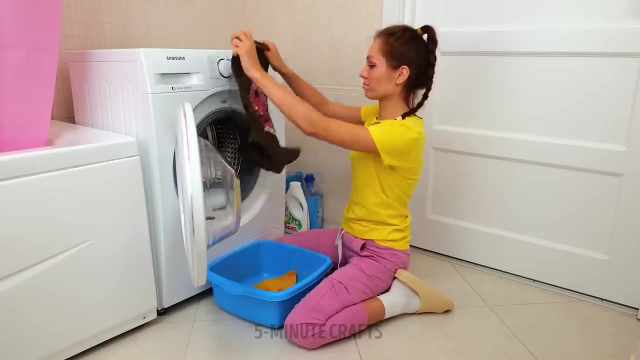 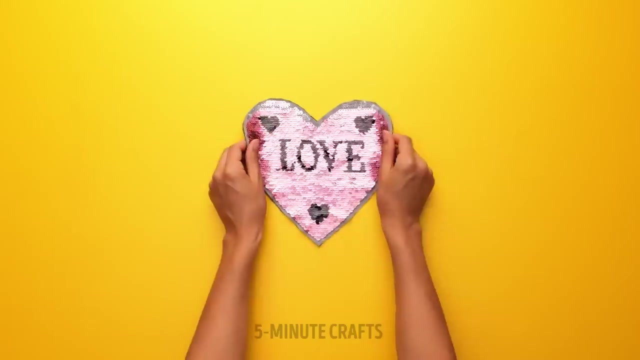 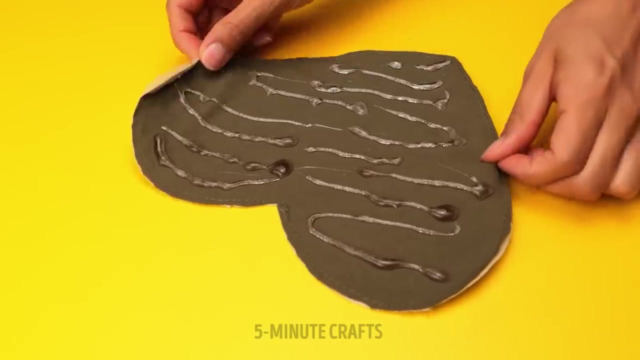 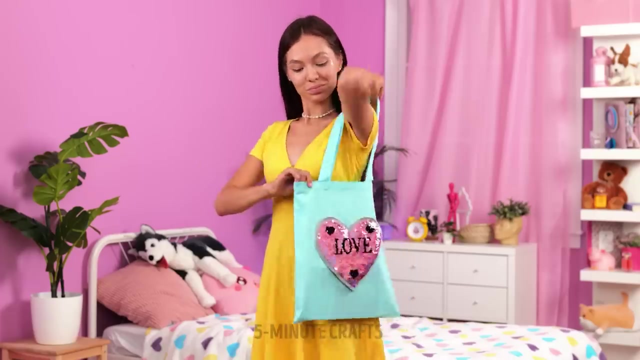 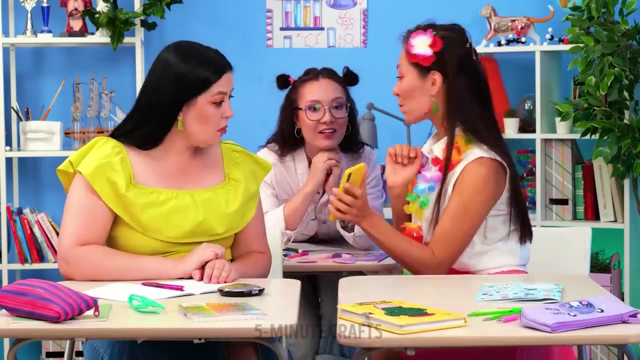 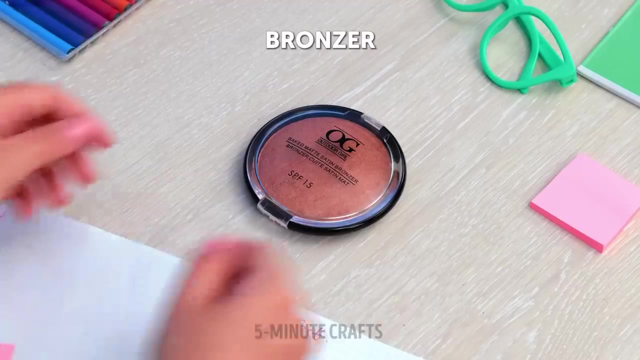 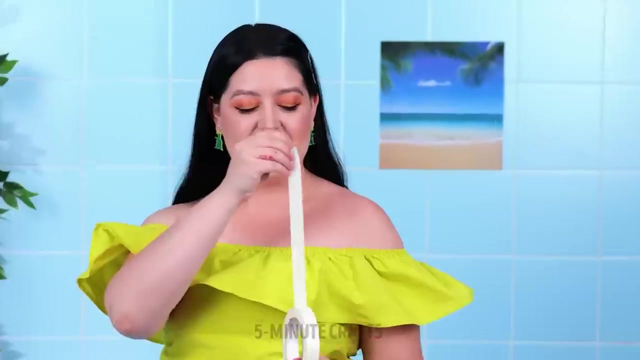 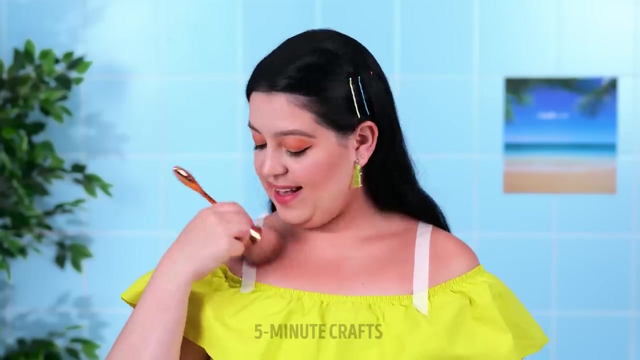 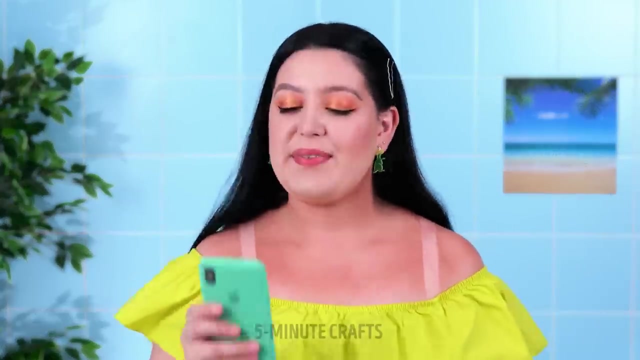 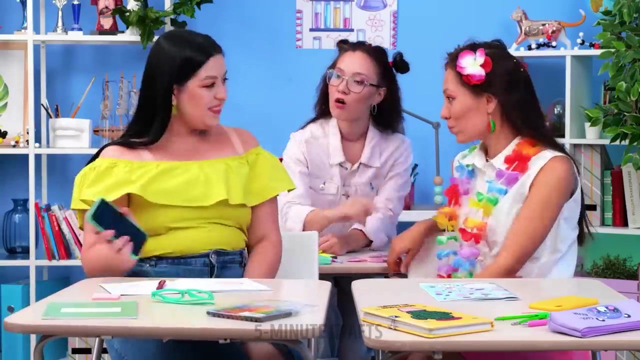 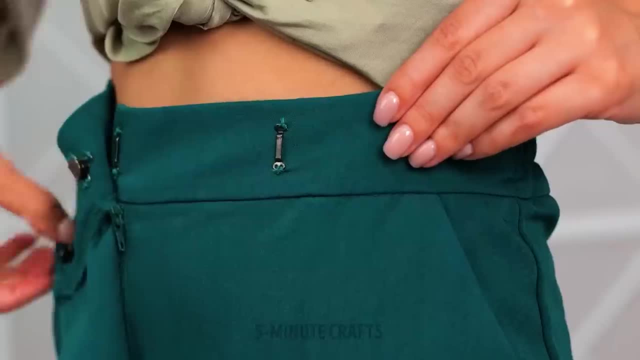 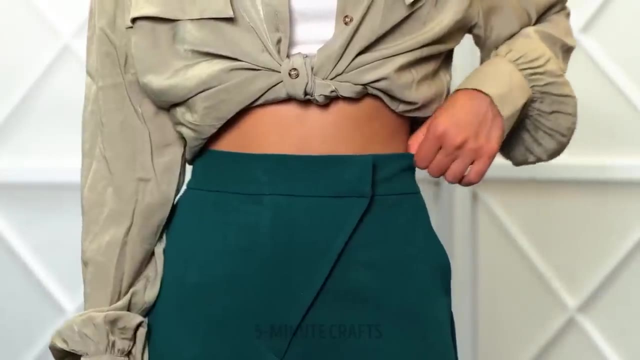 Me dijiste: no quiero nada, pero aquí eres toda mujer. Baby, yo te hago soñar algo más rico que la miel, Mi droga que te regalice. no digamos el pecado, Que hay cosas que no se dicen y en la piel te chocan. 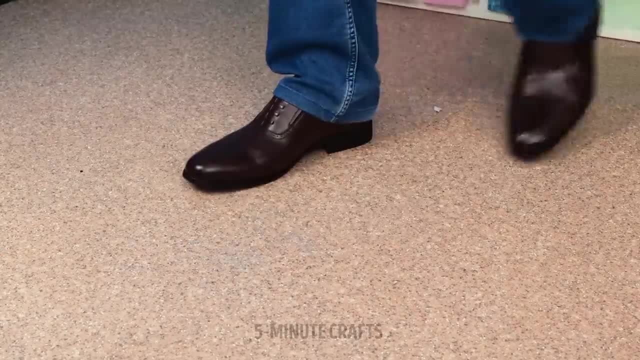 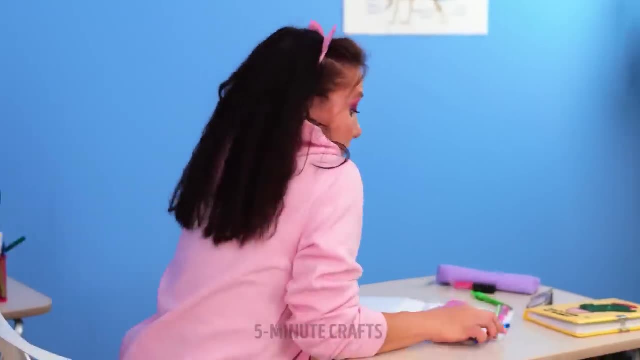 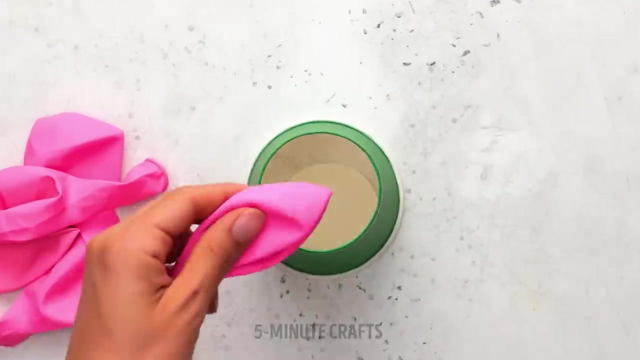 Baby, ¿para qué? te dices, Y tú solo dices que quieres más Que maten la curiosidad. eso es, Baby, si se nos da, será lo que será. Los dos vamos a matar toda esa curiosidad, Baby, si se nos da, será lo que será. 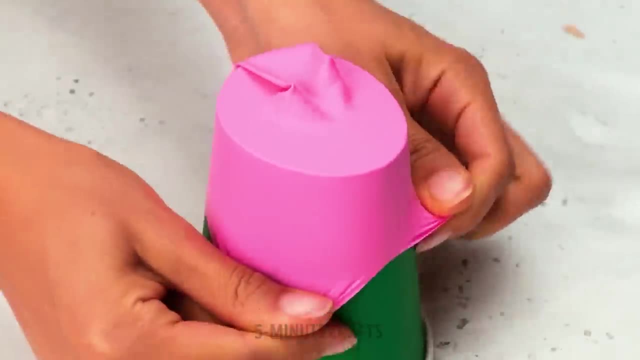 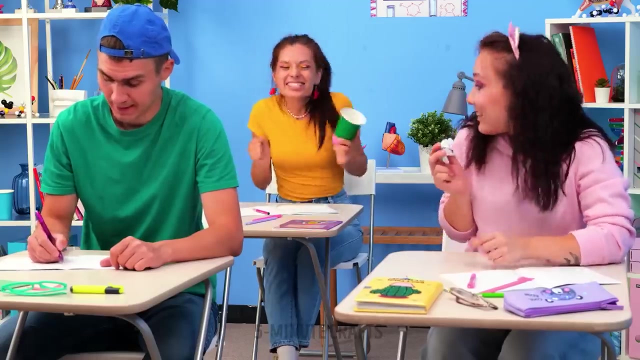 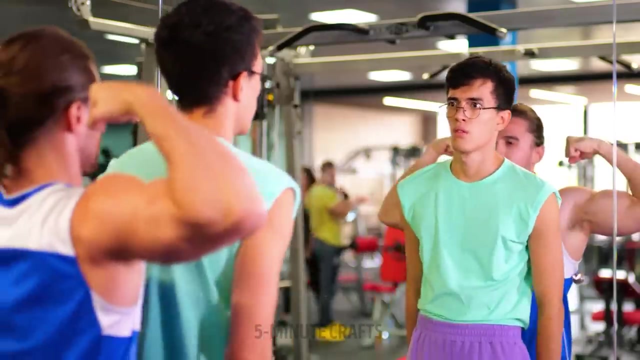 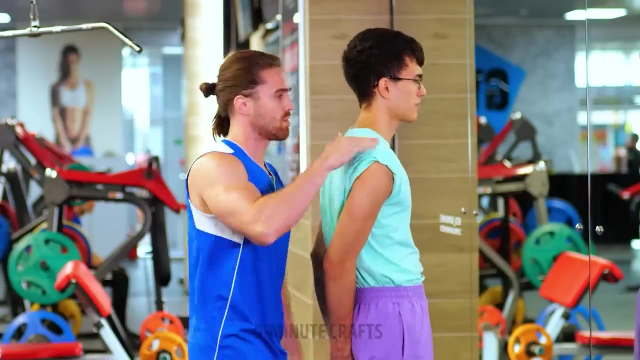 Los dos vamos a matar toda esa curiosidad, Toda esa curiosidad. Yeah, aquí viviendo Roche, Estamos solitos. eso mata la truce, Vengándote bien en todo, baby, para que tu creces. No somos algo serio, pero bien, si me conoces, 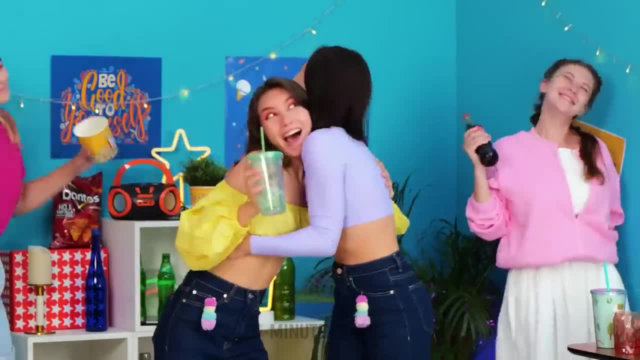 Yeah, yeah, tú eres el antojo de mi vida. Sin tanto que te pienso, ya no encuentro la salida. Pero no somos nada, nada girl. Pero no somos nada, nada girl, Baby, si se nos da. 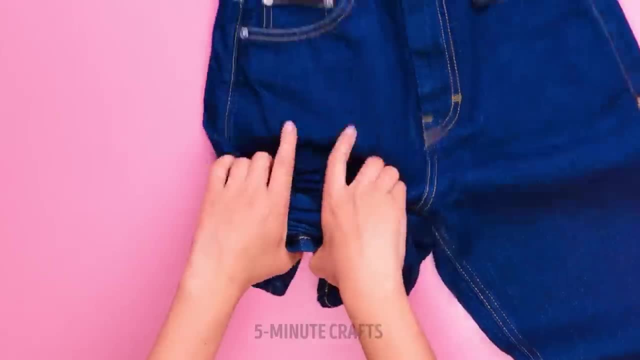 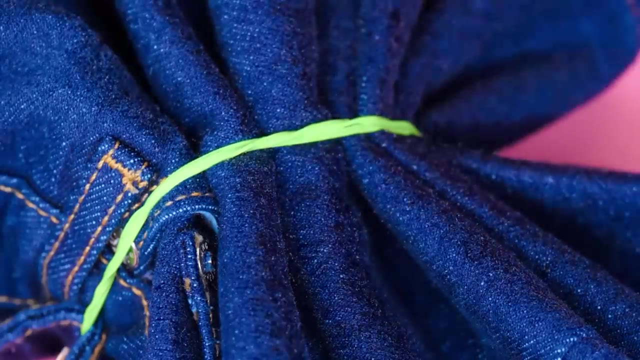 Será lo que será Baby si se nos da será lo que será. It will be what it will be. we are going to kill all that curiosity. But what if it doesn't happen? it will be what it will be. we are going to kill all that curiosity. 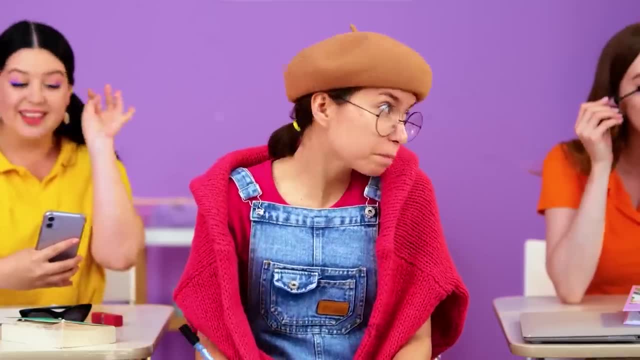 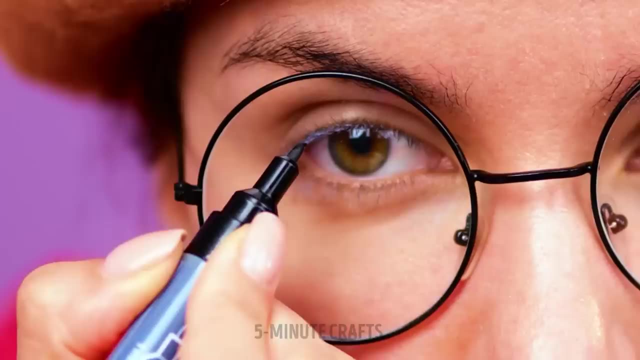 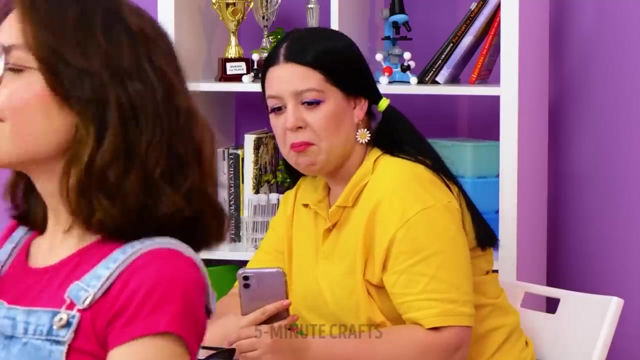 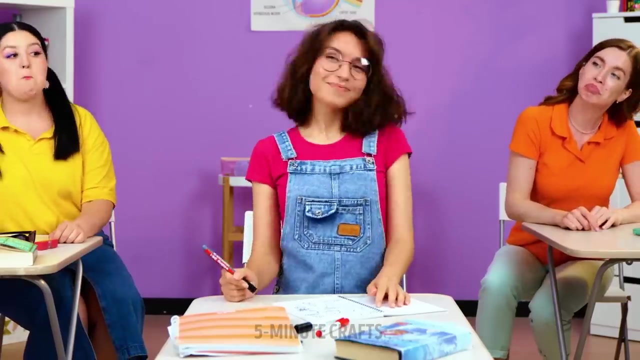 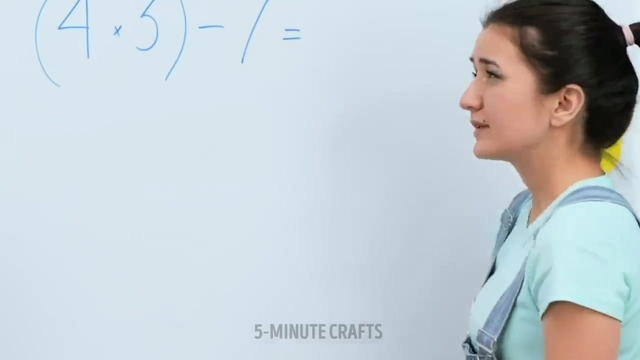 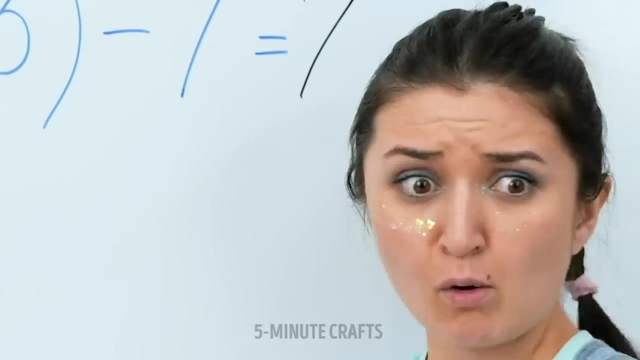 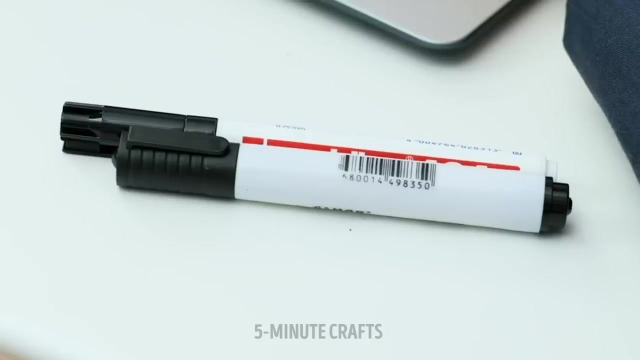 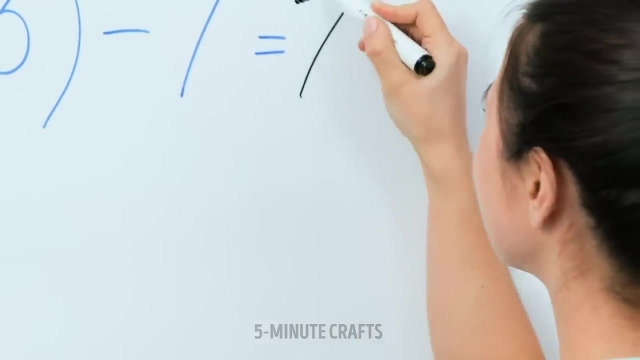 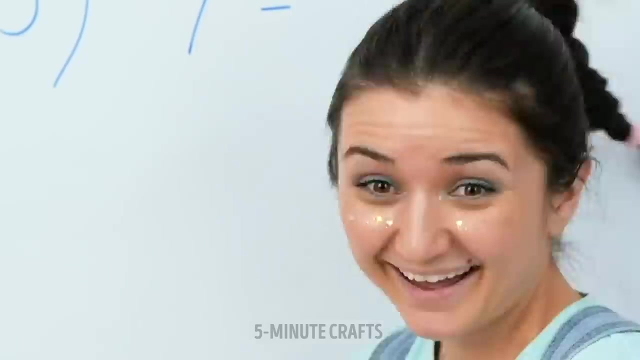 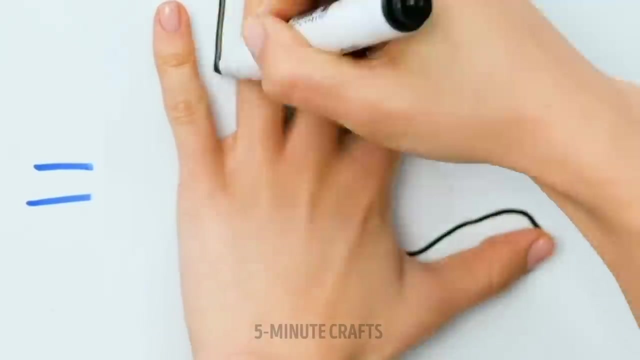 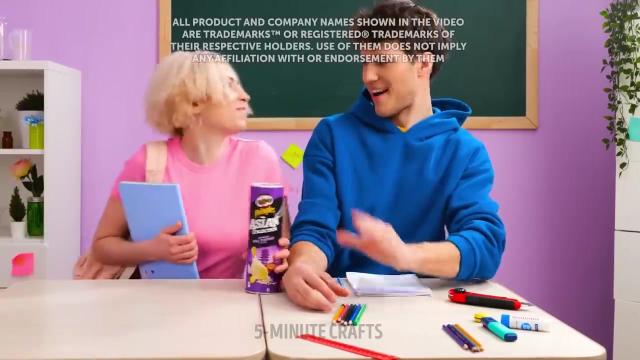 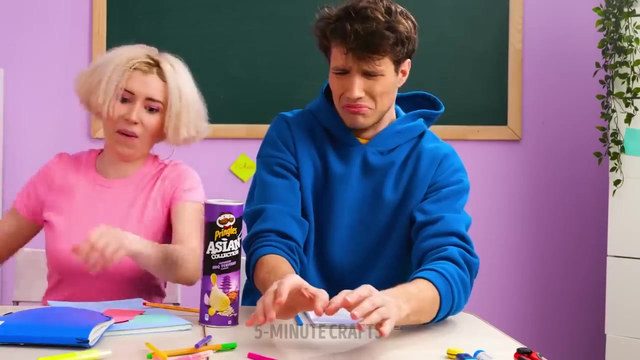 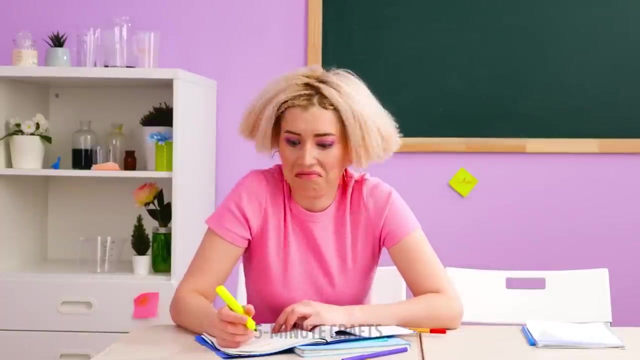 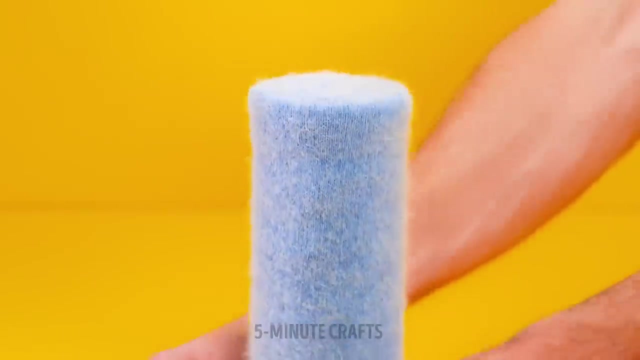 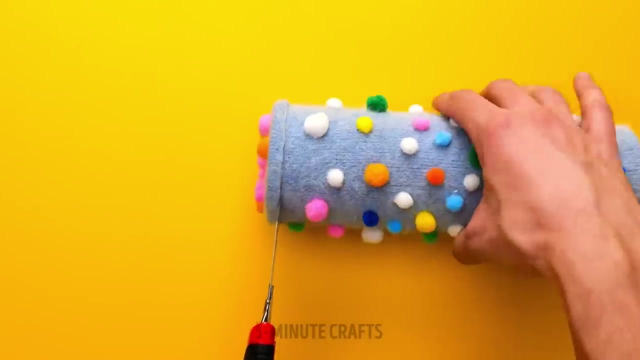 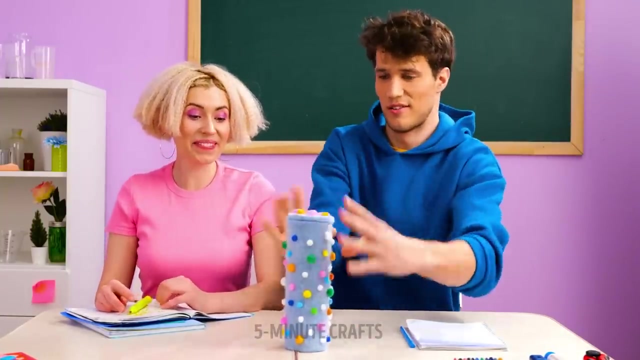 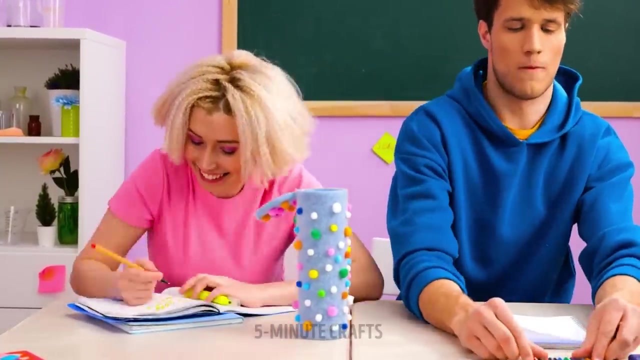 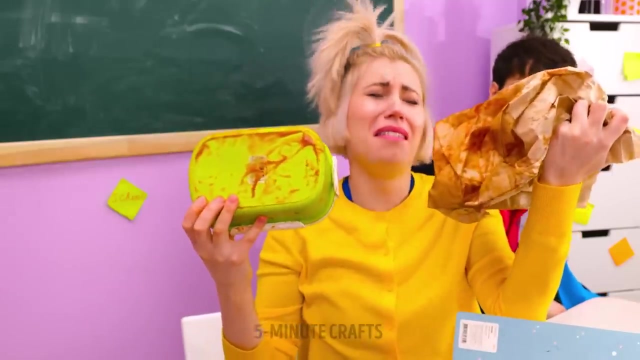 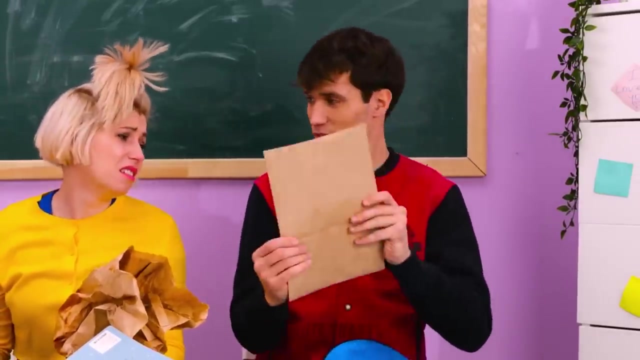 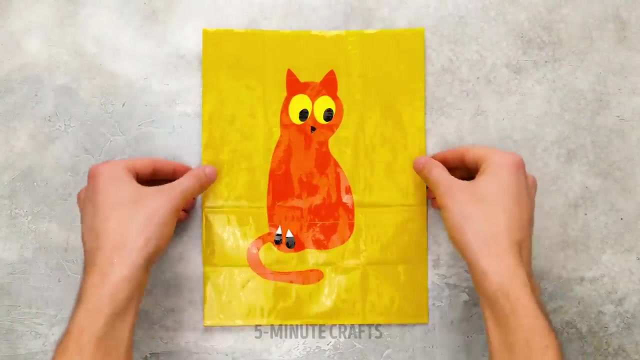 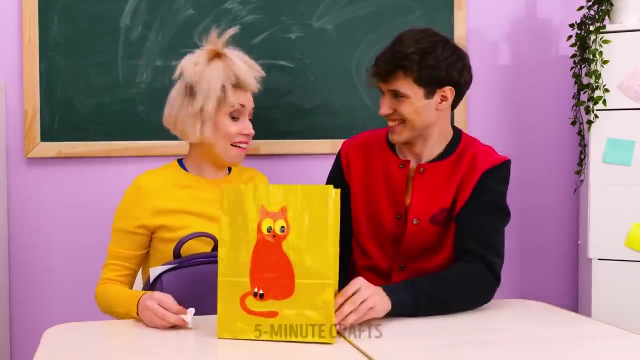 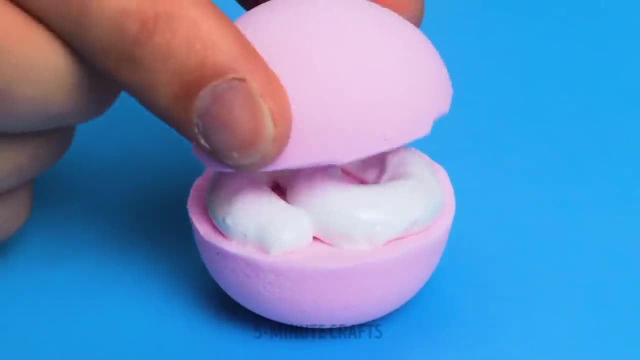 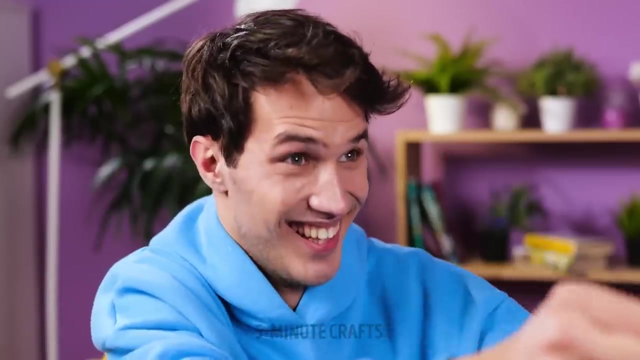 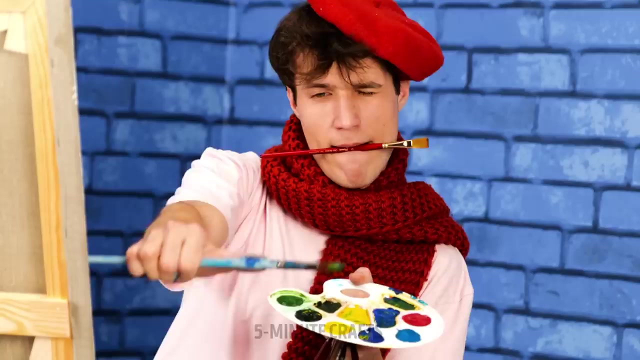 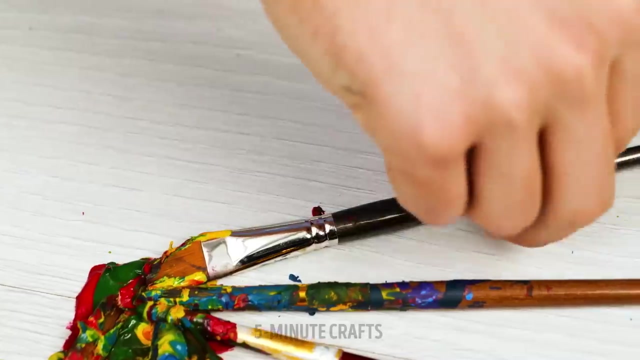 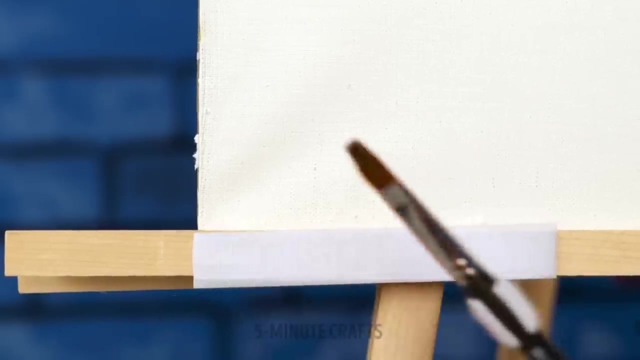 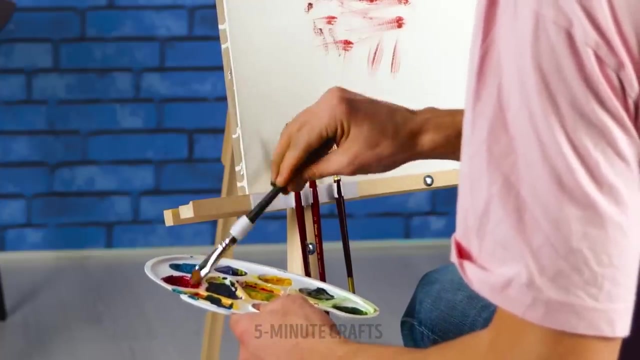 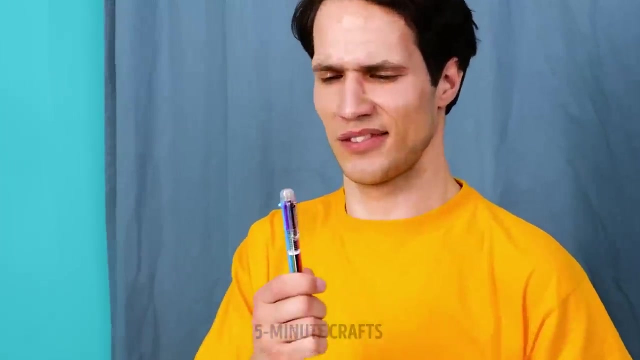 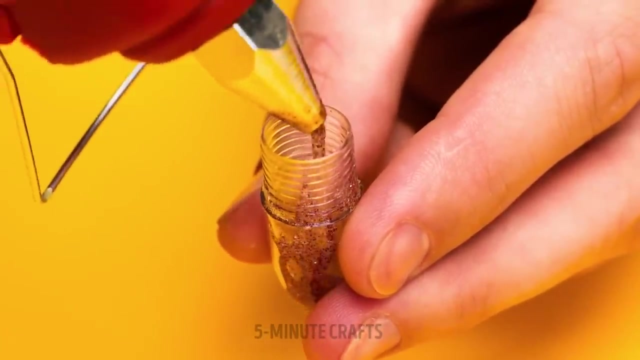 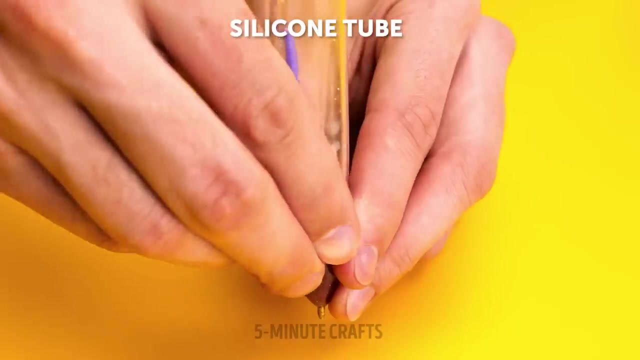 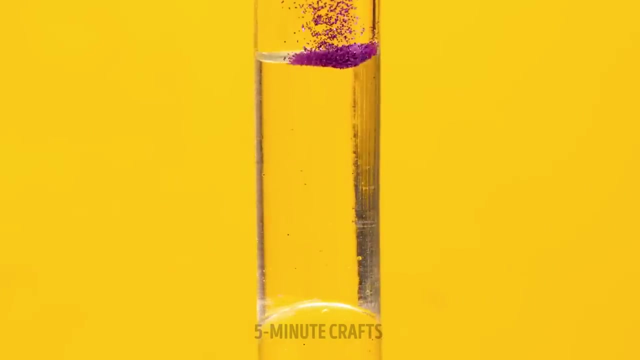 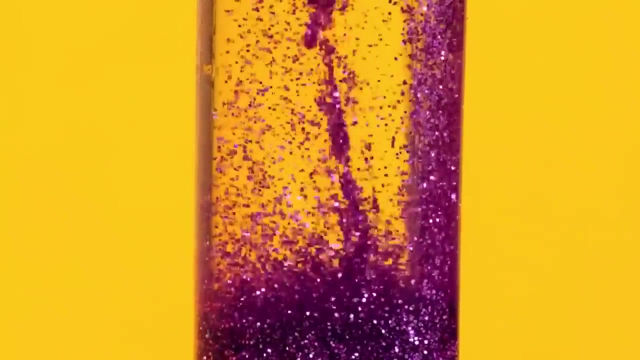 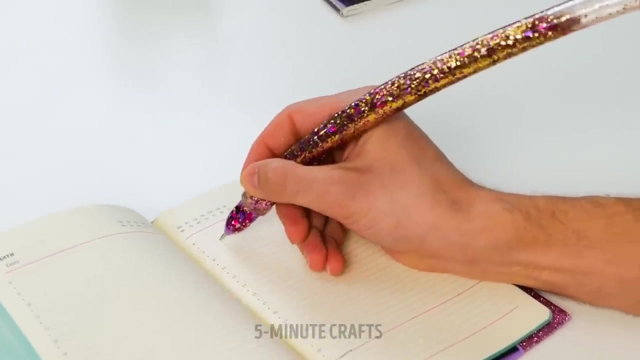 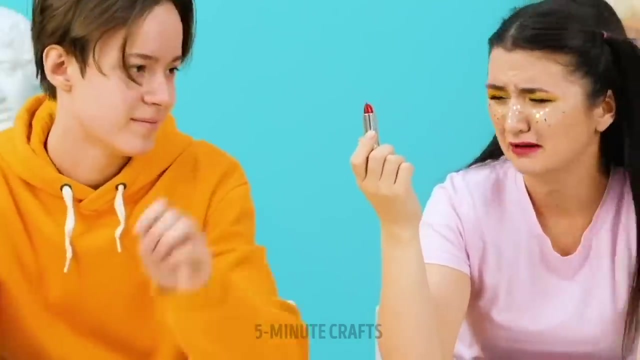 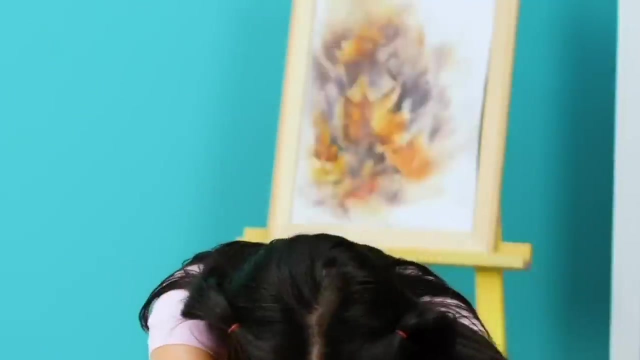 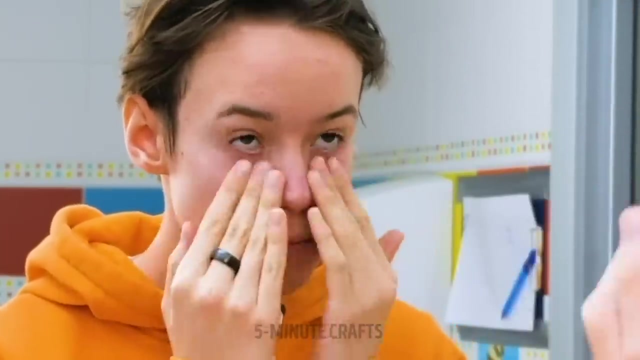 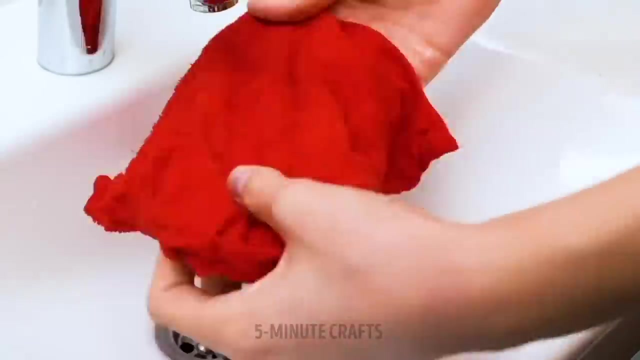 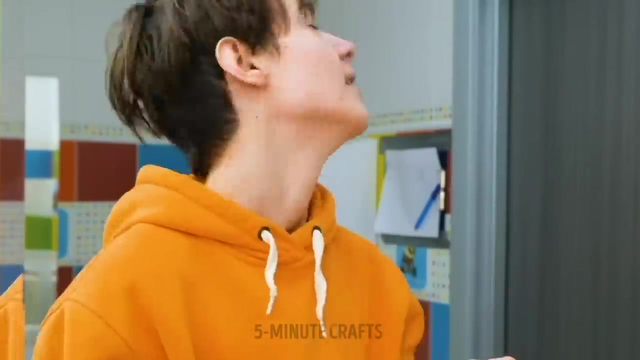 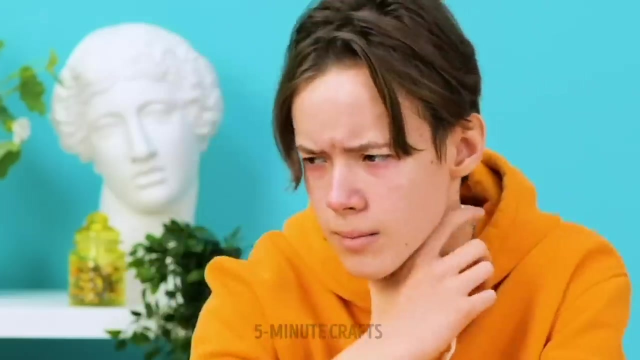 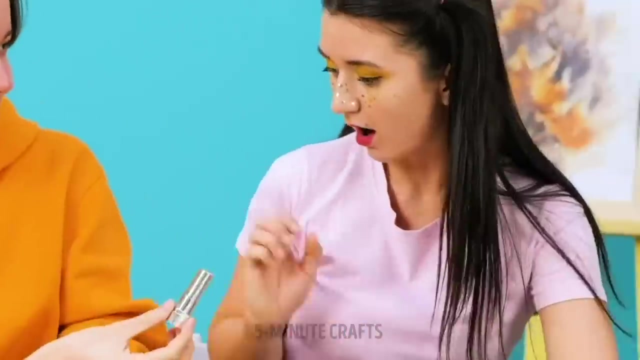 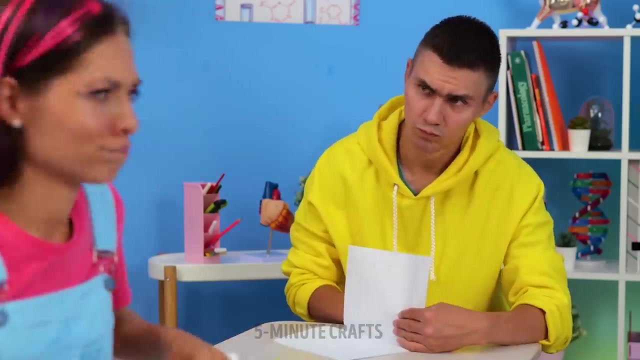 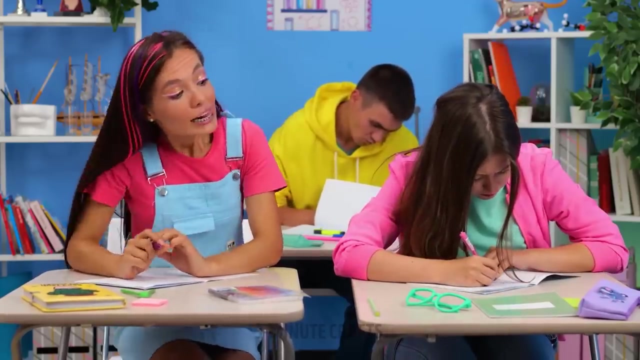 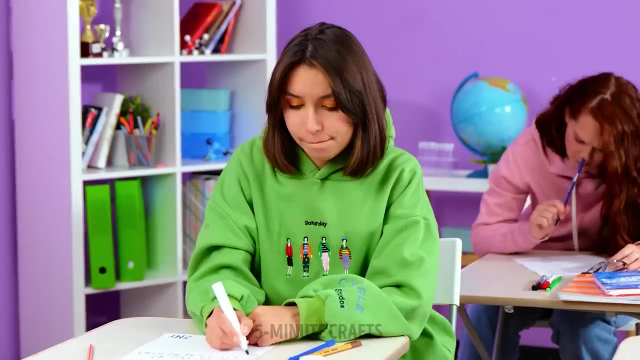 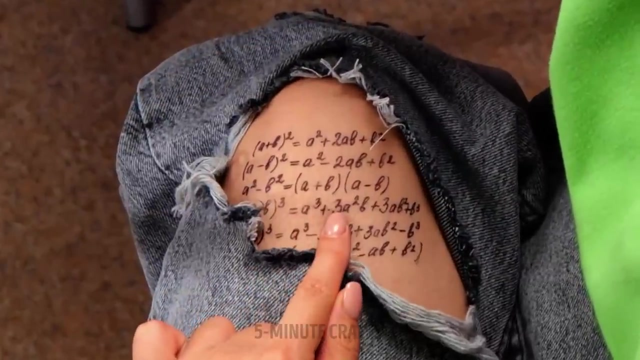 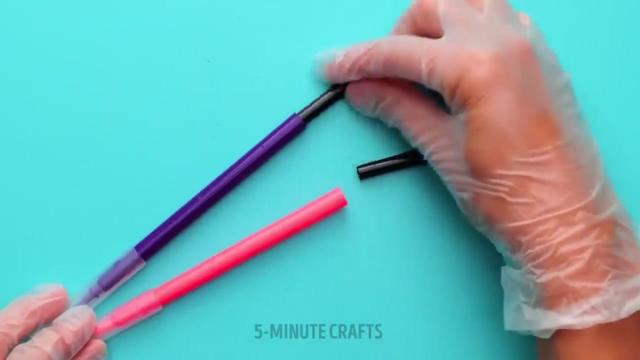 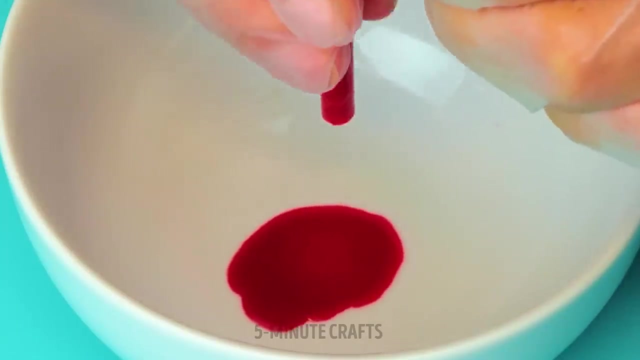 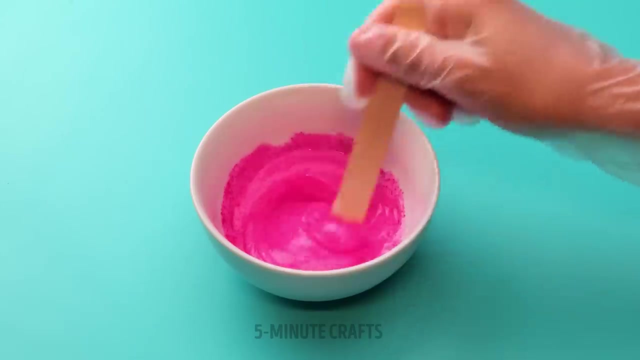 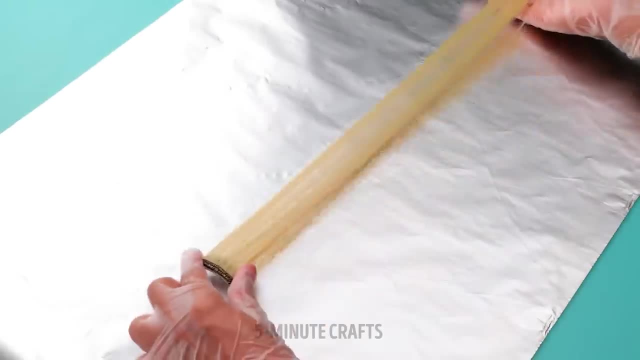 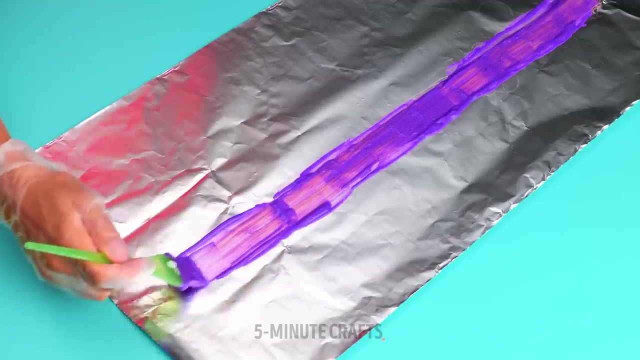 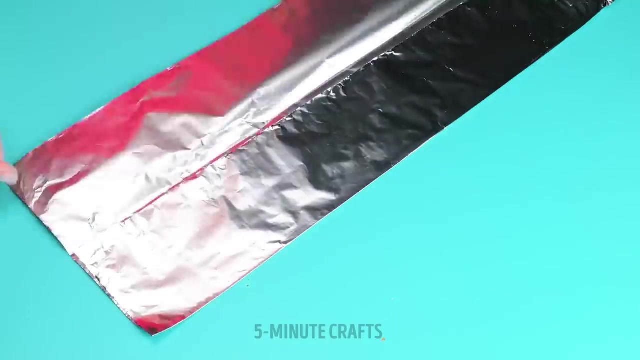 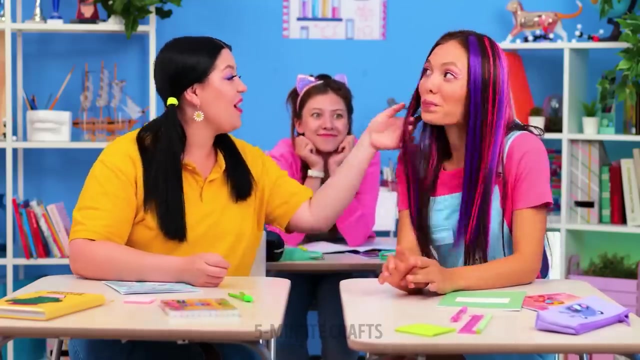 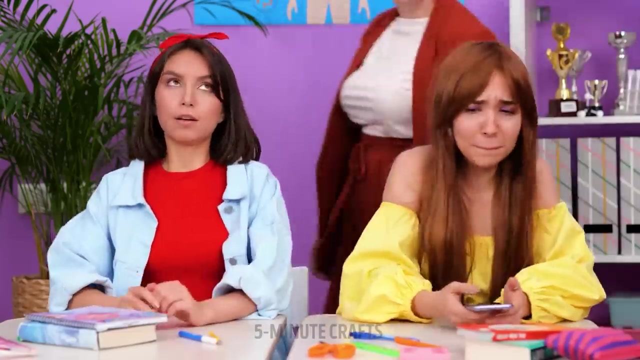 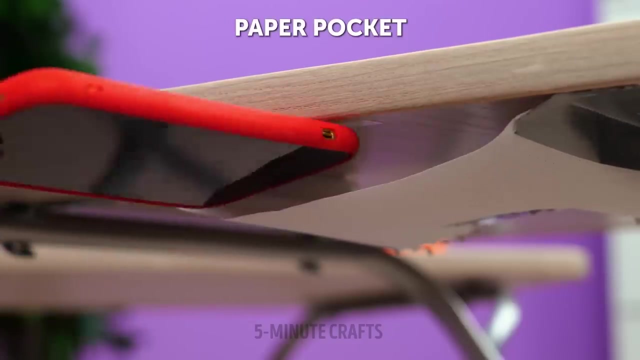 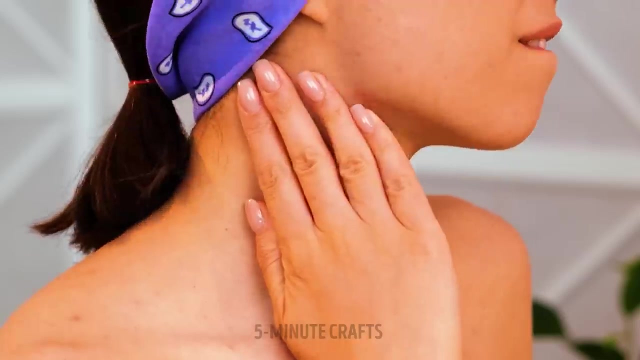 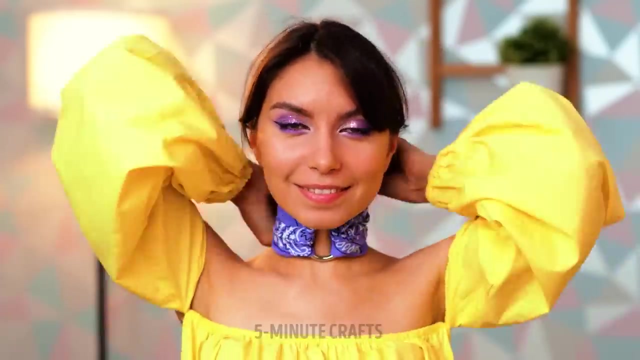 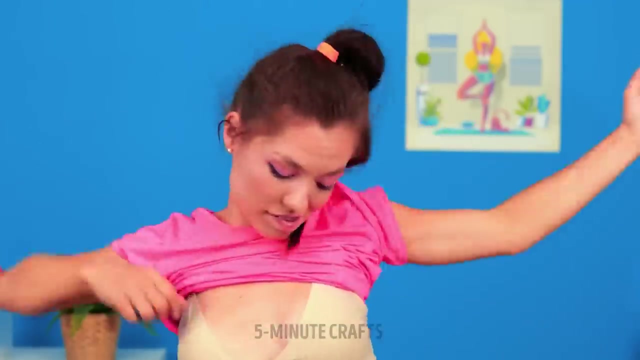 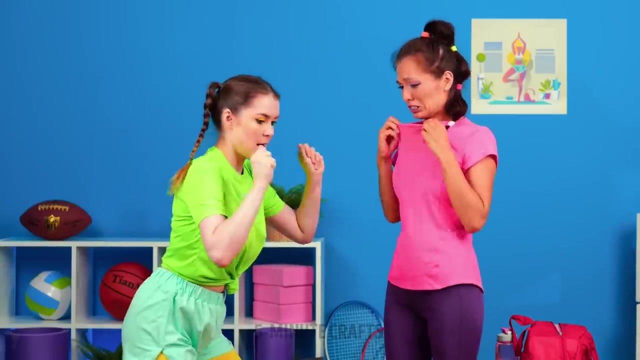 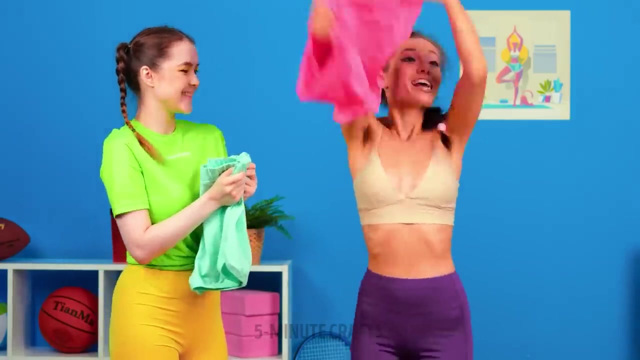 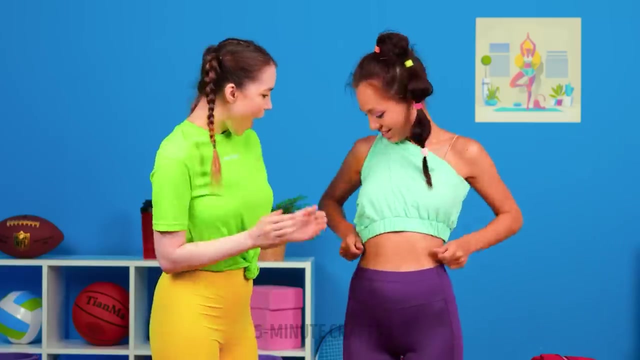 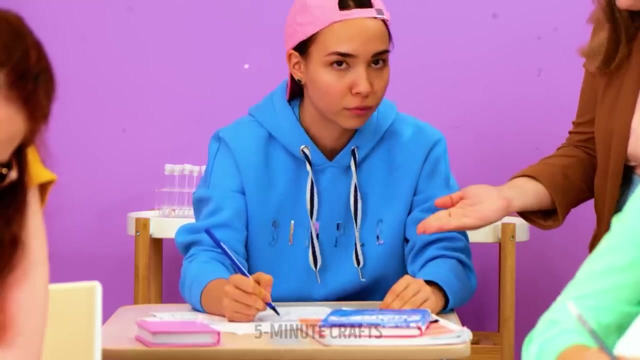 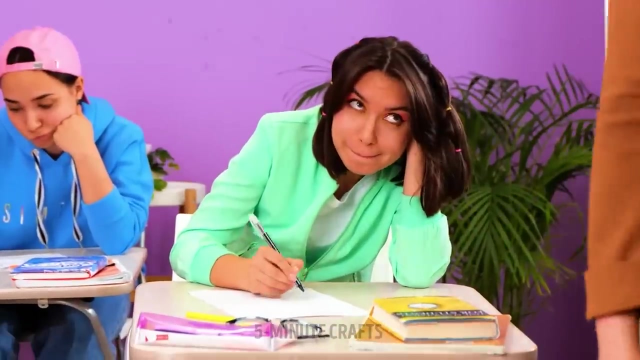 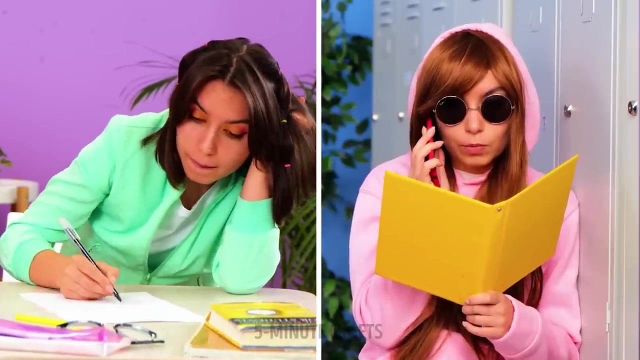 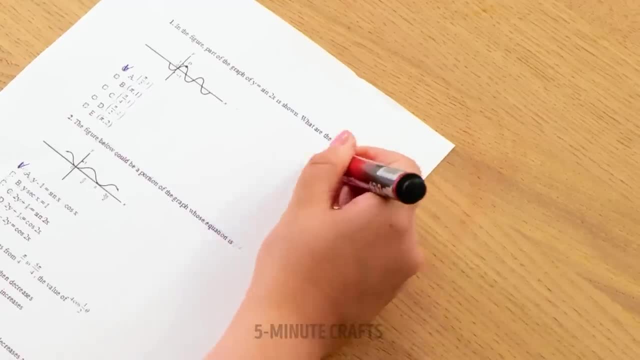 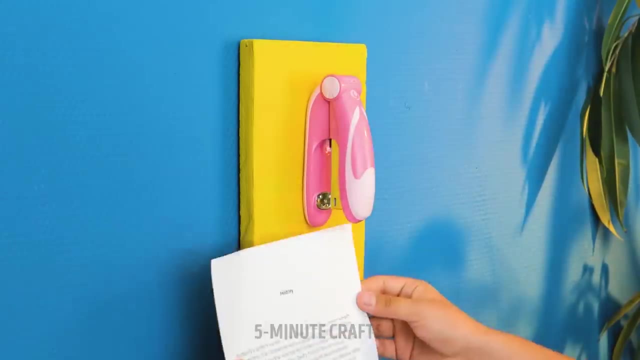 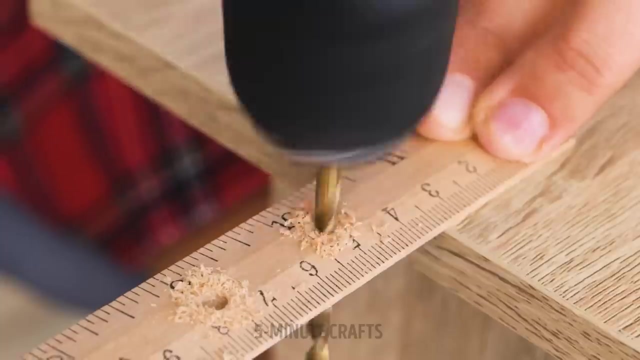 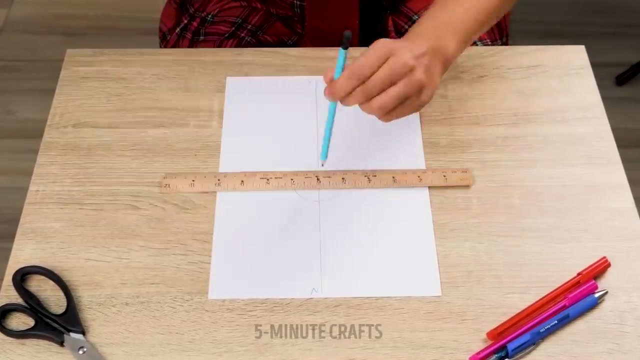 No, my body don't move like that. Don't make me pretend I don't see a shortcoming. You'll be running when I raise the black flag. Get out your bomb and fly away. We'll be dancing with our heads in the air When our new dawn is rising. 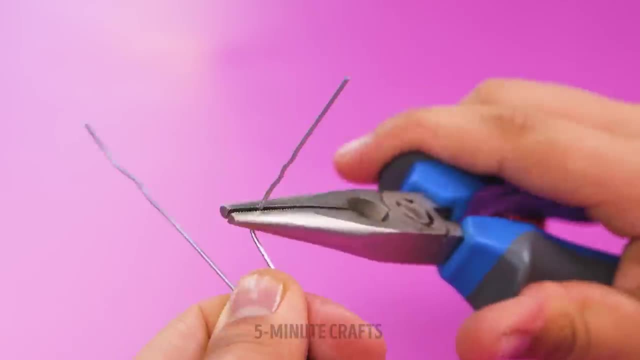 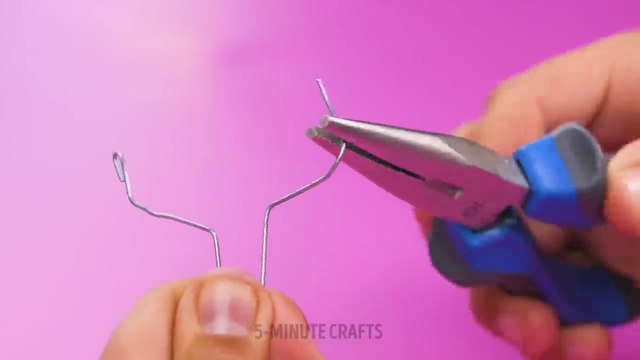 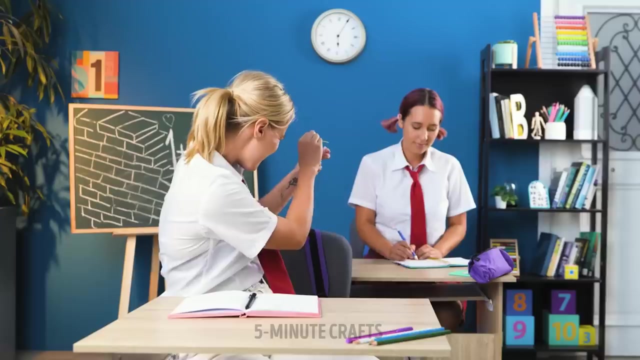 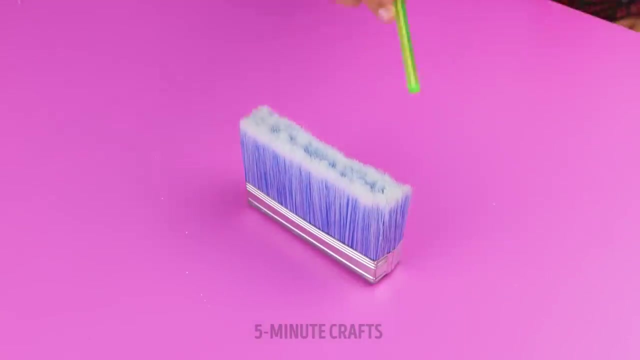 To the break of dawn. You can keep me in a cage made of tired ideas. It's a rush, and now I'm faster by the day. I won't wear your leash, I won't take no deals. I won't stay quiet when there's so much left to say.